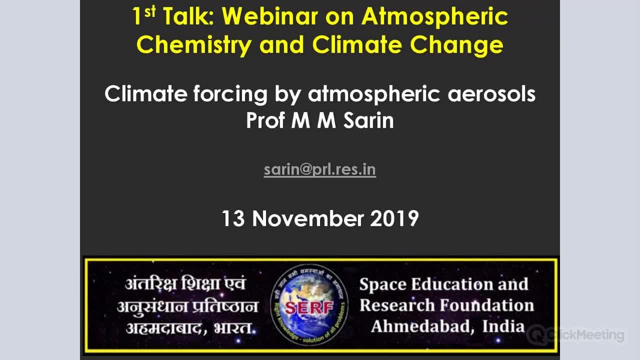 M Sarin had a very excellent academic and research career. at present He is a DST-SERB, Distinguished Fellow at Physical Research Laboratory and Honorary Scientist in Geoscience Division of Physical Research Laboratory. He did his MSc Chemistry from Nagpur University and 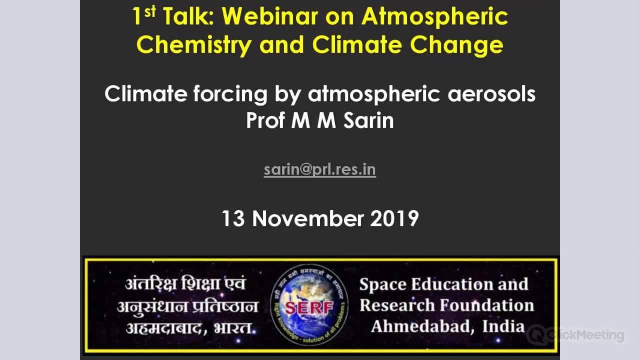 PhD at Physical Research Laboratory, Ahmedabad, which is a unit of Department of Space He had. he joined PRL and worked at several academic positions And in 2013, he retired as a senior professor And since then he has been Honorary Scientist and the Distinguished 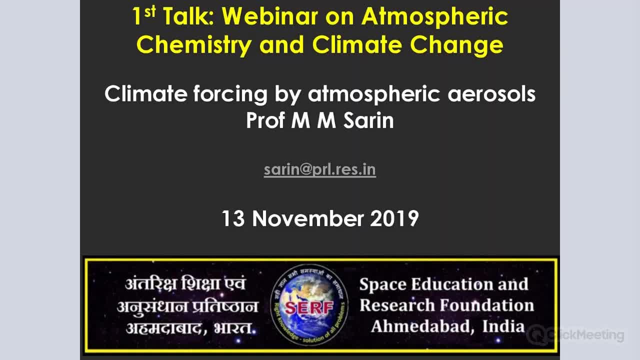 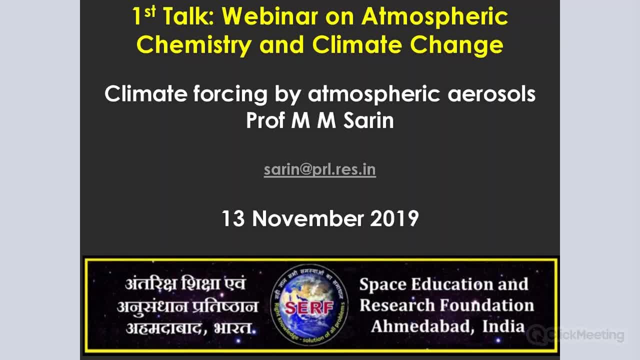 He has published 155 research papers in refereed journals. He is a fellow. there are three science academies in India and he is a fellow of all three of them. He has served as project director of ISRO's geosphere biosphere program on atmospheric and mineral dust. atmospheric mineral dust. 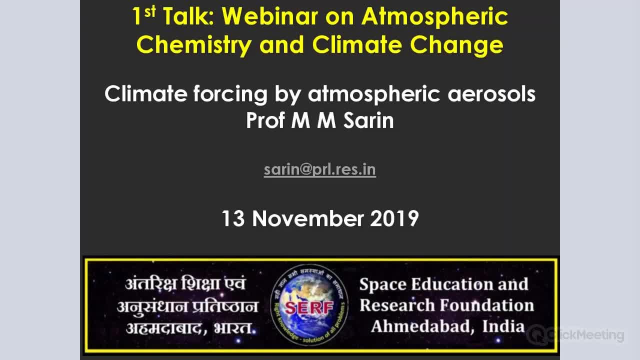 He is a member of the International Commission on Atmospheric Chemistry and Global Pollution. He is also a member of the Scientific Committee on Oceanic Research. He has served as a visiting professor at Woods Hall Oceanographic Institute, Massachusetts in the USA, and Ocean Research Institute of Tokyo University. 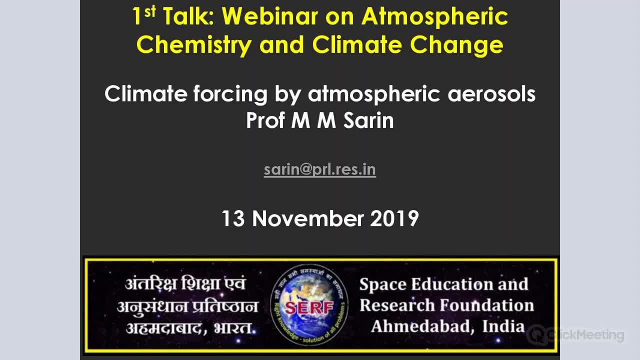 Currently, he is the vice chairman of the United Nations Group of Experts on Scientific Aspects of Marine Environmental Protection. With these few words now, I request Professor Sarin to deliver his talk, and we all will enjoy listening to him, Professor Sarin, please. 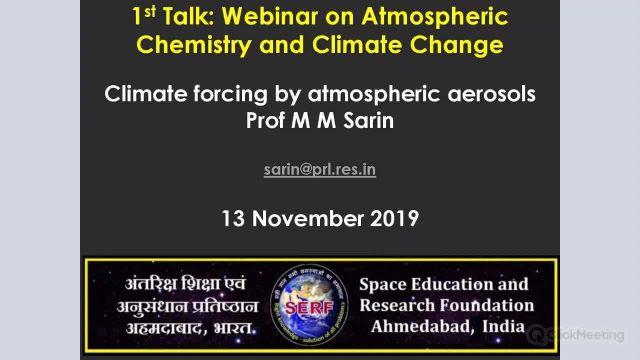 Very good morning to all the listeners from Ahmedabad, India, And I would like to discuss some basic concepts on the climate forcing by atmospheric aerosols And in the next three talks I will further elaborate the concepts on the various constituents of the atmospheric aerosols. 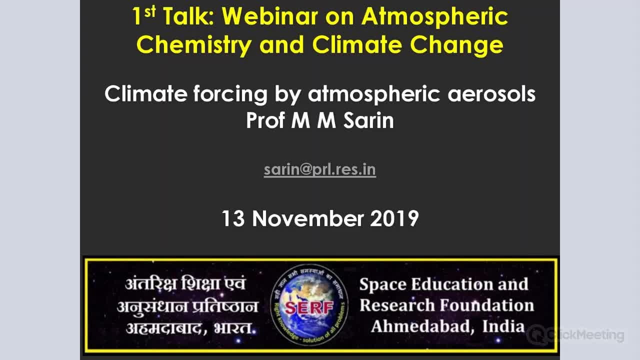 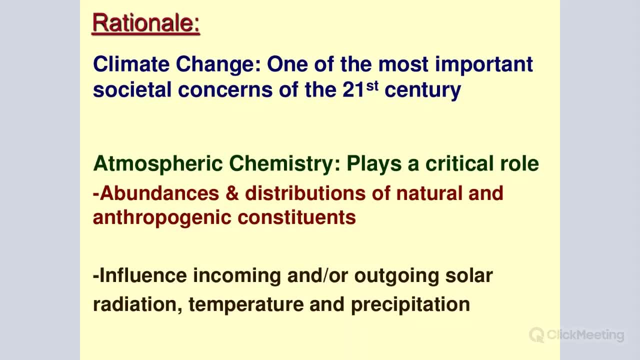 So I would like to briefly address this issue: How the climate change has become the most important societal concern in the 21st century, And this is one of the most debatable points in the present day context, because of the anthropogenic activities which all of us are responsible for it. 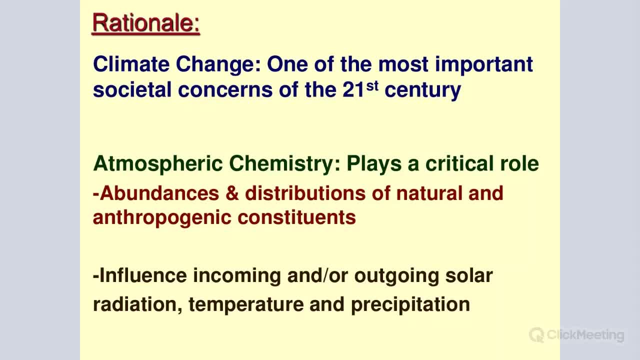 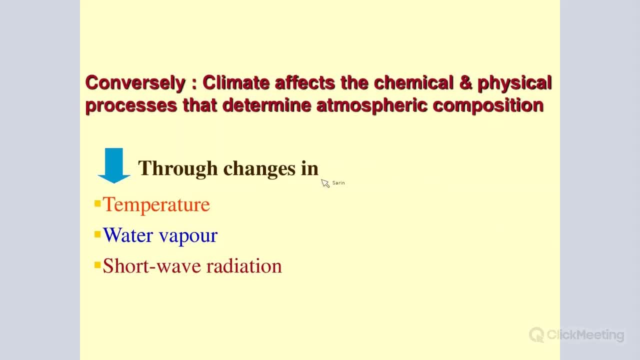 And in this context the atmospheric chemistry plays a very critical role and that is largely in the climate change. And in this context the atmospheric chemistry plays a very critical role and that is largely in the climate change. largely happens through the changes in the temperature and water vapor and the incoming 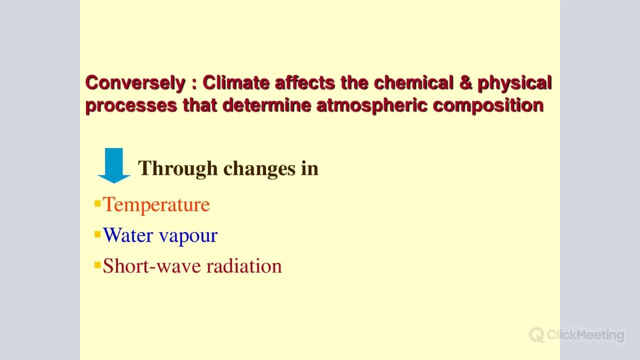 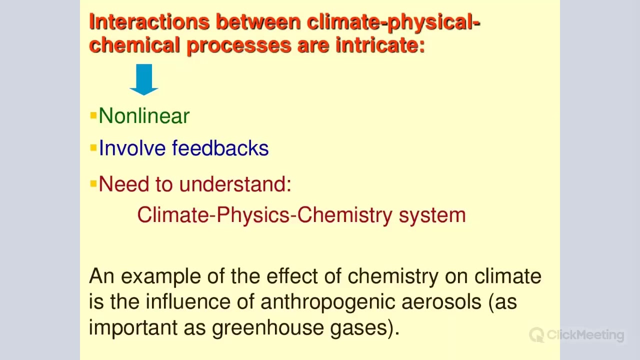 shortwave radiation. So these are the main factors which are responsible for the climate affecting the physical processes as well as the atmospheric composition. So in this context, it is also now relevant that the interactions between the climate, physical and chemical process are very intricate, because we have to understand all the three. 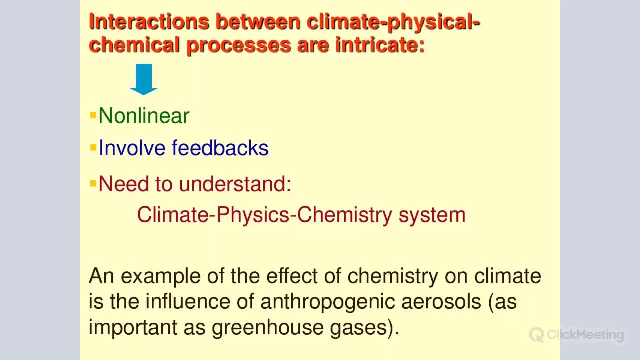 systems together: Climate, we have to understand. we have to understand the physical processes, we have to understand the chemical process and these are, of course, very intricate. and basically they are intricate because of the nonlinear behavior of these processes. they involve the feedbacks which I will discuss in this talk. 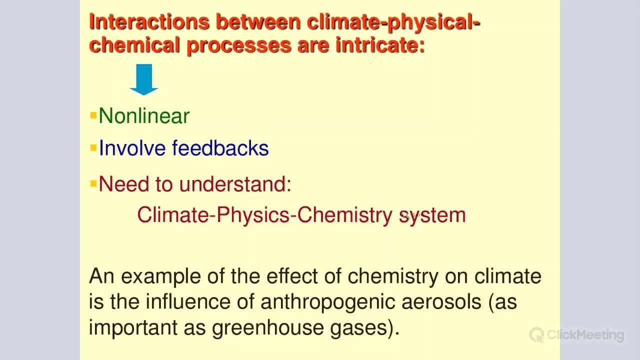 So we need to understand the climate physical processes, But if we understand the characteristics of these particular aspects in a holistic way, then we can only try to understand how the aerosols and the atmospheric chemistry are going to have the influence on the climate change. 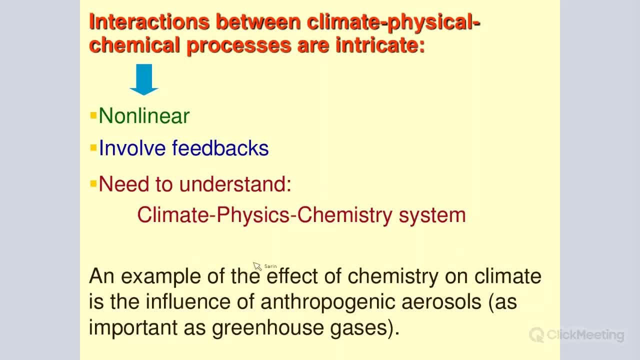 So one of the very simple examples of the chemistry or the effect of chemistry on the climate is the influence of the anthropogenic aerosol, as important as the greenhouse gases. So I am not going to go into much of the greenhouse gases, because greenhouse the warming potential. 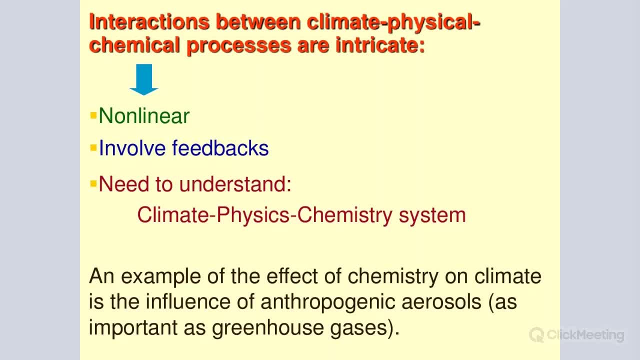 has been well understood. But I think the main thing is that it's not just about the greenhouse gases, It's about the carbon and carbon nesse in the, in in the recent years, but the, uh, the warming or the cooling effect by the, by the 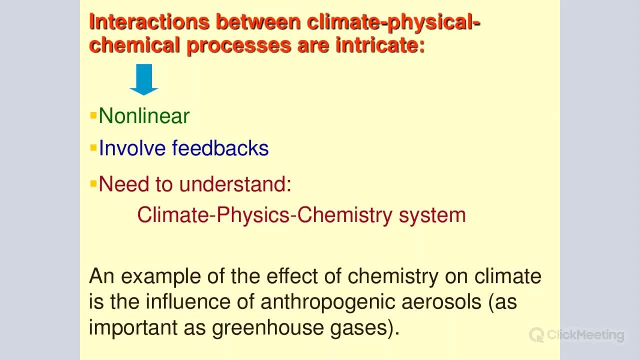 aerosol is something which is more debatable, and that's where the the present day efforts are going on to understand how the anthropogenic aerosols are going to uh, cool or or warm the atmosphere. so, but this is as important as the greenhouse gases, because green greenhouse gases 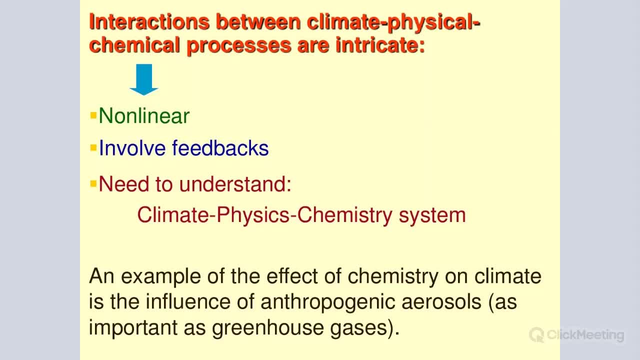 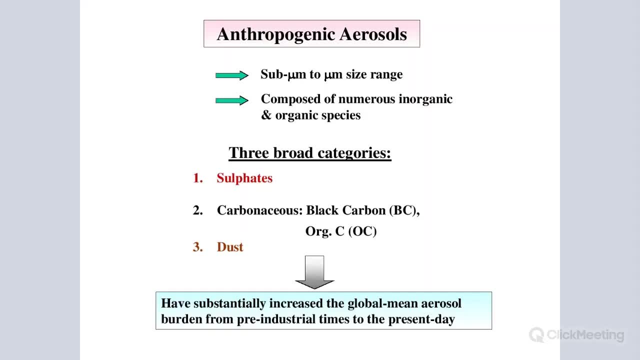 are are being much understood, that the they are causing the global warming. so this we, we, we know in in this aspect. so so let us see the, see the, the anthropogenic aerosols. now, what are these anthropogenic aerosols? these are are primarily in the sub micron to micrometer size range, and 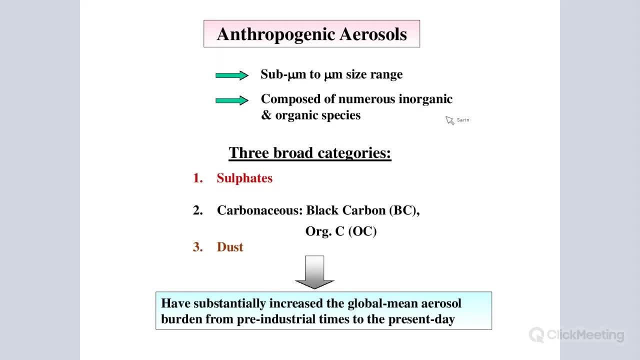 they are. they are composed of of numerous inorganic as well as the organic species and they can be broadly classified into three categories. one is the sulfates, which are coming from both the natural and the anthropogenic sources, mainly now from the anthropogenic sources, because sulfates are being added from all the industries and various other other. uh, commercial, uh, the. 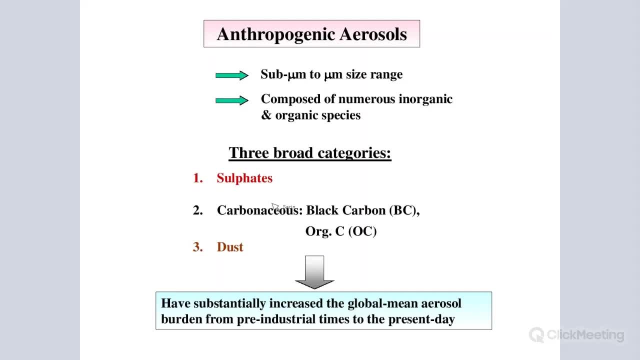 agencies. and then we have this carbonaceous aerosol, which i will deal separately in a in a talk tomorrow, and these consist of of primary, the black carbon, which we we refer as bc, and then the organic carbon which is uh referred as the oc in in the subsequent uh uh. 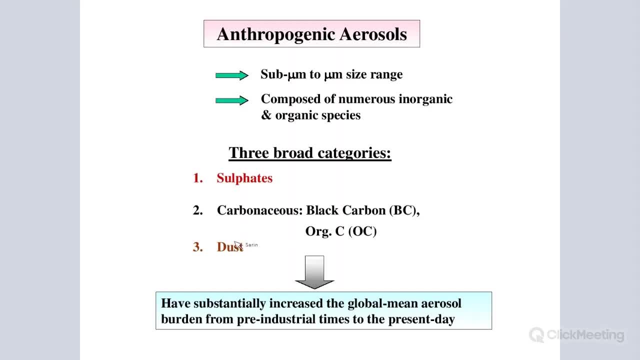 talk, and then the most important thing is the dust, which is third constituent of the of the atmosphere. dust is a perennial constituent in the atmosphere, so we have to understand the role of dust also in the in in the climate, as well as in the chemistry scenario. so dust is a, is a very 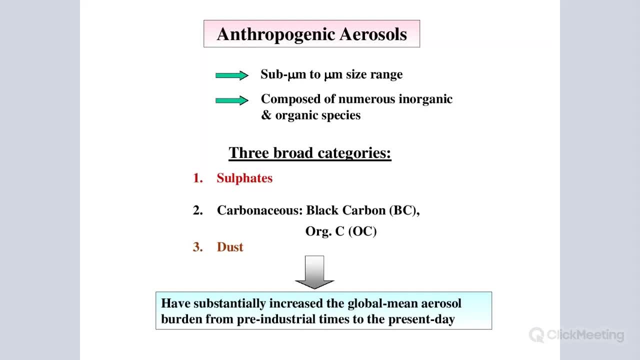 potential uh constituents and i will. i'll deal with this dust also in a separate talk uh day after tomorrow. so so what? one has to keep in mind that if that the anthropogenic aerosols which we are, primarily the sulfates which are coming from anthropogenic sources, some of them are from from. 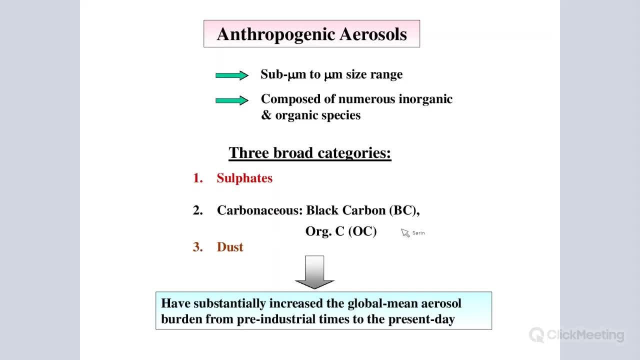 natural carbonaceous are largely coming from the biomass burning fossil fuel, as well as the coal burning and dust, as i said, is a perennial constituents and present in the atmosphere and and also being added by the various other anthropogenic activities. but natural dust sources are very important. so these, uh, these constituents have increased the global mean aerosol burden. 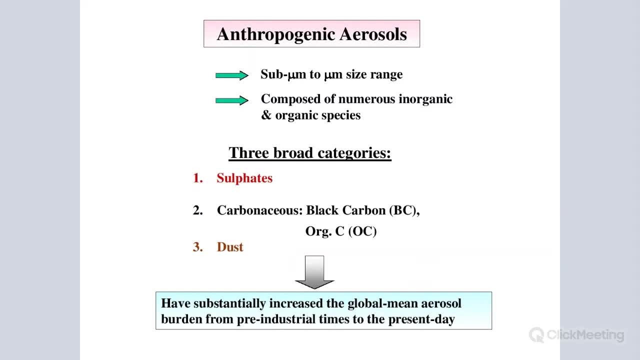 from pre-industrial time to the present day. this is very important. so one has to keep this in mind- that in the last 200 years uh, the concentration of sulfates, carbonaceous aerosol dust, in constant in the atmosphere has increased substantially, and that is the reason for the uh, for the cause. 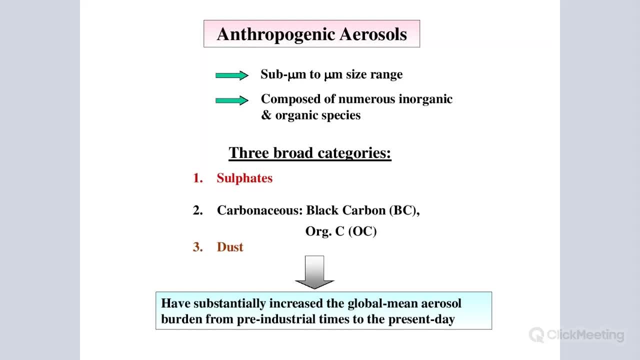 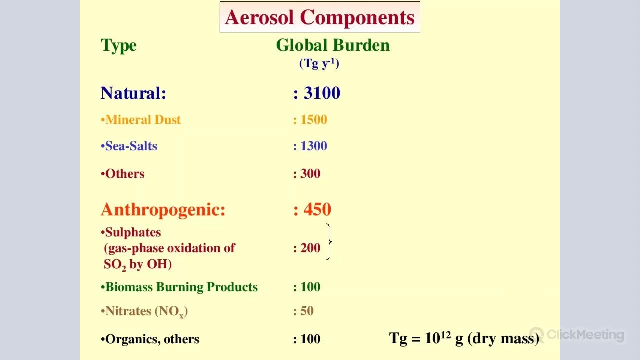 and the debate or the concern that how the atmosphere chemistry is going to change in the in the context of these uh, these type of anthropogenic aerosols, and what are the influences is going to have. so so let us try to understand further. what are the uh? are the simple aerosol components which 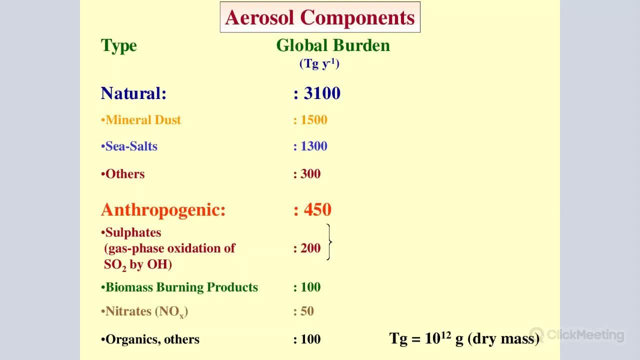 we are talking about, as i said in the in the previous uh, uh slide. so, uh, there are. there are three, uh, there are, uh, there are two types, which i will uh, i will dwell upon. one is the natural and these are the. are the units in terragrams per year. this is the, the global burden. uh, as of. 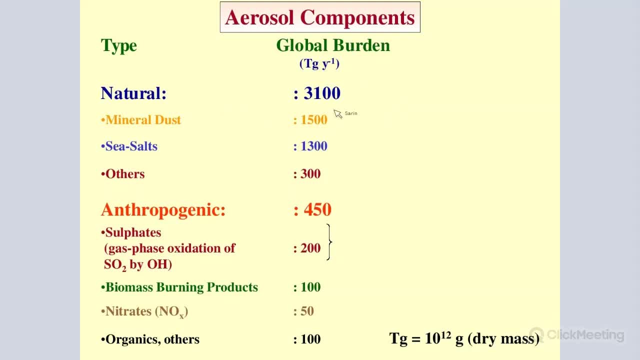 today. so you can see that the in the in the natural law, of the order of of 3100, the anthropogenic are about 450 and in the natural context we are basically talking about the mineral dust, sea salts which come from the marine, because, uh, oceans cover the large surface. 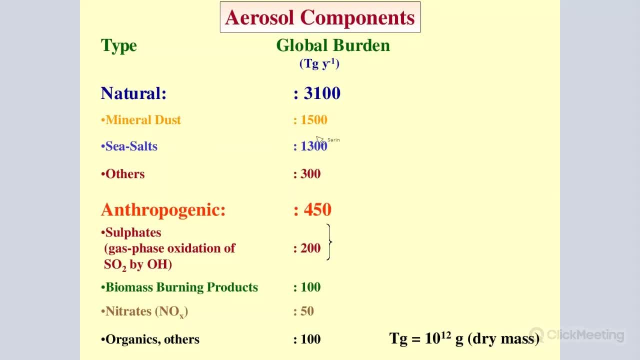 of the of the of the earth. so we have the, the sea salts and the others contribute uh to to some small level. so these, these are the, are the constituents which are, are are important in the, in our context, of the natural aerosol which have been there from the time immemorial. 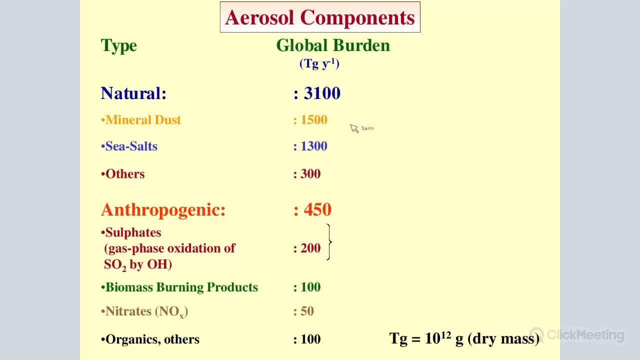 that the the natural, uh, our aerosols are part of the atmosphere and they are part of the atmospheric chemistry and they are part of the of the climate change now, once we we get into the anthropogenic aerosols. so these are having a burden of about 450 as of today, or close to 500. 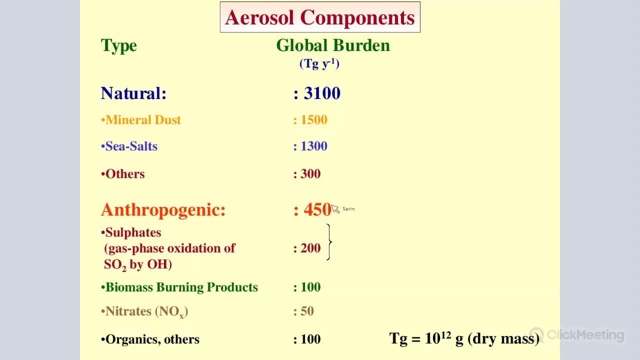 compared to your natural layers. so they are. they are still about not as as high as as a natural but, but nevertheless it is important to see that they are included in the atmosphere, and so this is is critical in the atmosphere. so the sulphates are basically coming from the from the gas phase oxidation of sulfur dioxide by the oh radical. 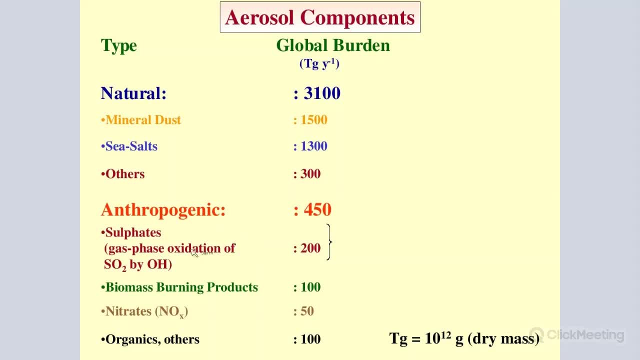 oh is very important in the atmosphere, because whatever we put in the in the atmosphere as a sort of pollutant that gets oxidized by the oh so, and sulfur dioxide is one of the. the anthropogenic constituents comes from the man-made activity. of course there are natural. 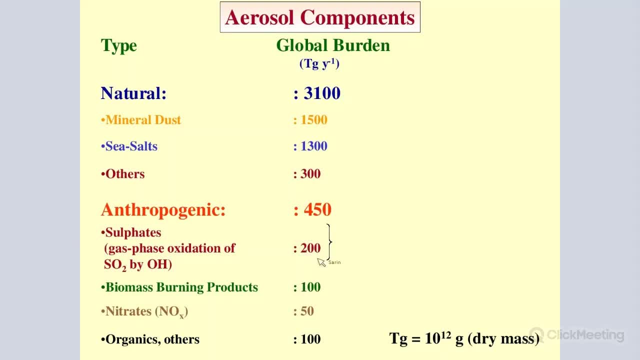 sources also, like volcanoes and those, but, but we are context, we are trying to address on the, on the gas phase, oxidation of sulfur dioxide, which is coming from the anthropogenic sources, and that is gets oxidized by the oh radical, because oh is, the is the most oxidizing agent in the atmosphere. so so that is one aspect. then we have the biobas burning. 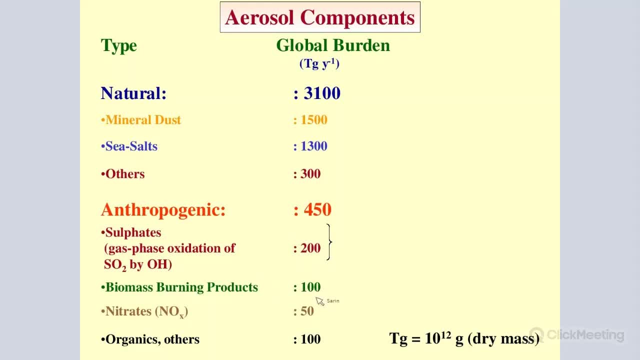 products which i told you in the previous cell about the black carbon and the organic carbon, and they are also adding substantial amount of of of aerosol constituents in the atmosphere. next comes the, the nitrate, and then we have the, the other organics, which are also important. so these, these, 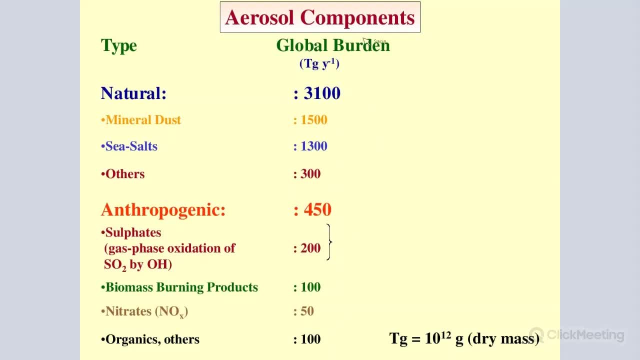 all put together, we have the, have the aerosol components which are present in the, in the, in the atmosphere. so this is what we have to have to understand, and we see that the what, how we understand the, the impact of these, both natural as well as the anthropogenic aerosol in the climate. 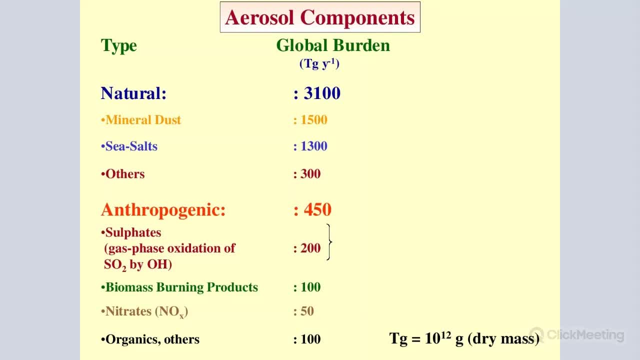 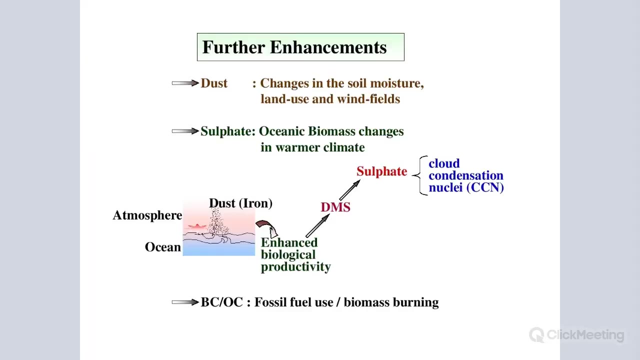 change scenario. but having said that, i i i made a very clear statement that the uh, that the uh, the global warming by the anthropogenic greenhouse gases, is well understood, so i will not go into those details in this particular job. then then what happens to these these uh, both natural as well as the anthropogenic aerosol? so further enhancements are expected. this: 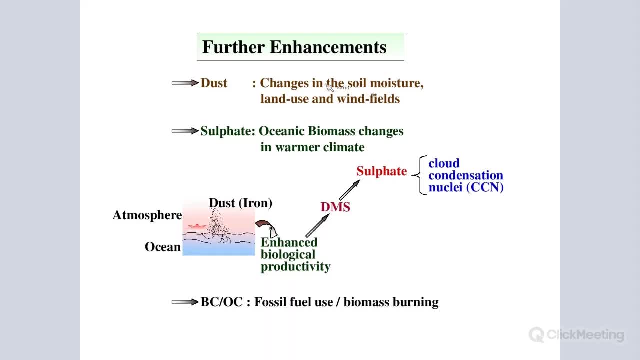 is something which is very important and that is for the dust, because of the changes in the soil moisture that again depends on the precipitation rainfall, so the, if soil moisture decreases, then you will have more suspension of dust in the atmosphere, as well as the land use and the and the other, uh, the, the wind fields which are going to change. 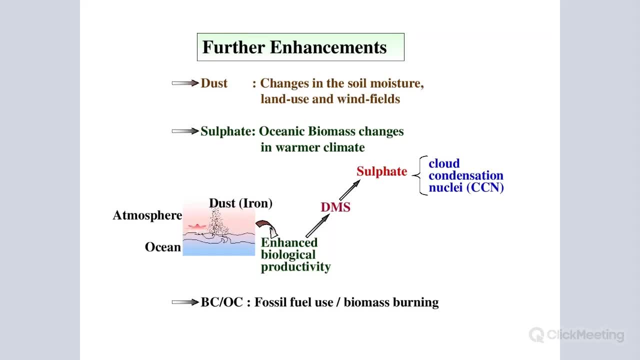 so and you have the long-range transport of dust from the desert regions as well as from the other anthropogenic land use cover change, so these are all going to have the further enhancement of these, of the of the dust. sulfates are, as i said, are coming from the uh, the anthropogenic sources in 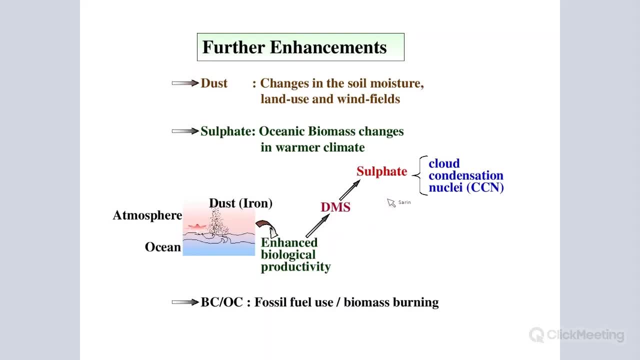 the forestries and then- but there is a very important and perennial source of sulfate- comes from the, comes from the oceanic biomass and that is because of the, because ocean has the, the primary productivity by the. and if, if primary productivity increases in the ocean, which the efforts have been, 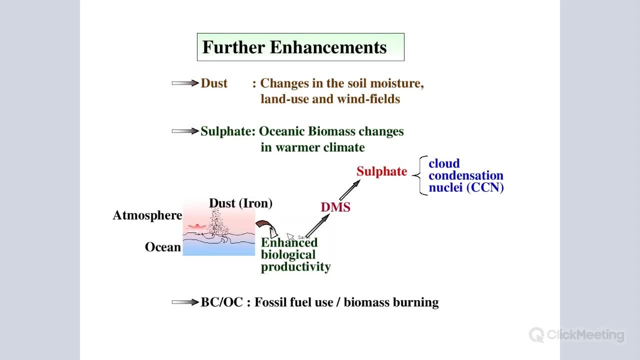 tried. i will discuss on this aspect in my in my fourth talk. uh, if dust is being added from the atmosphere, that means basically iron is being added from the atmosphere. so iron acts as a micronutrient for the and has a very important role in the development of the environment. so that is. 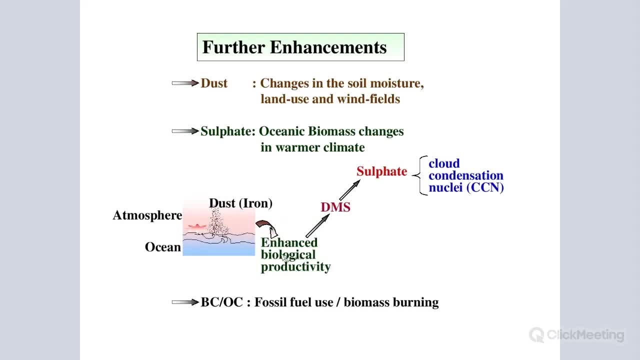 a very important role in the development of the environment. so that is the, the biological productivity in the ocean, and the biological productivity enhances. then you produce more of our dimethyl sulfide, which is a gas which is uh, and, and that gets finally oxidized to sulfate and that sulfate acts as a cloud condensation nuclei. i will address 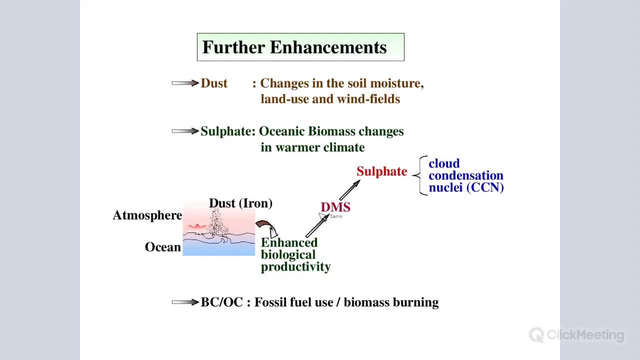 this uh particular aspect of ccn, how these are. so there are uh not only the um, the sources of uh, of sulfate coming from the industries, but it is also important to see that the, the, how the oceans will also can enhance the sulfate uh contribution in the atmosphere through this. 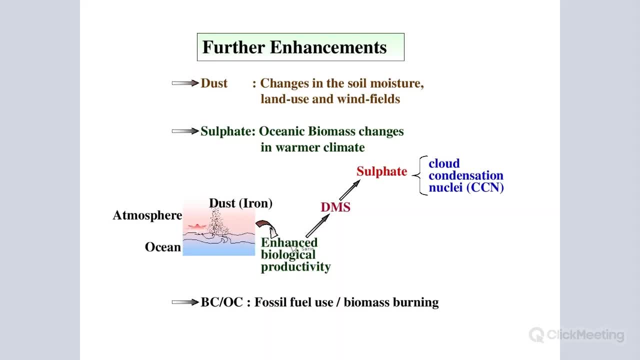 kind of biological changes in the uh, in the ocean, as a consequence of the of the climate change, or vice versa. if the, if the oceans are matting, so that will have impact on the climate change, or the climate change is there, then the ocean will will behave in a different way. so it's a, it's a. 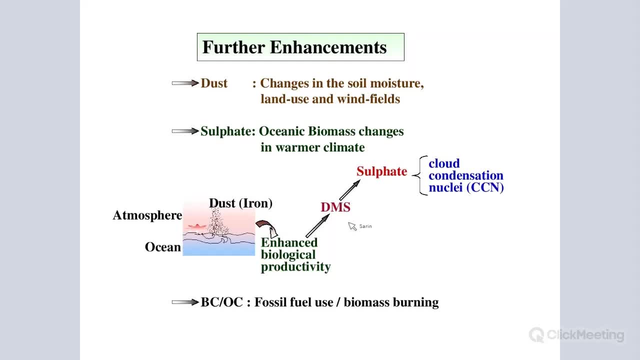 feedback, as well as the, as the, as well as the interactive uh system, and then, of course, the last aspect is the is the black carbon and nitrogen, as well as solar energy. also, uh nineteen, very long, is carbon, and the organic carbon which is coming from the fossil fuel, as well as biomass burning. 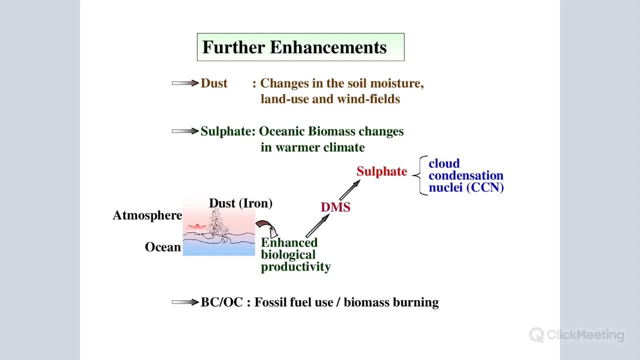 and coal burning. Coal burning is more original, so to say, and it is significant, but it is not significant for organic carbon, but it is certainly significant for the black carbon, But the fossil fuel is a major concern on the worldwide use of diesel petrol, so most 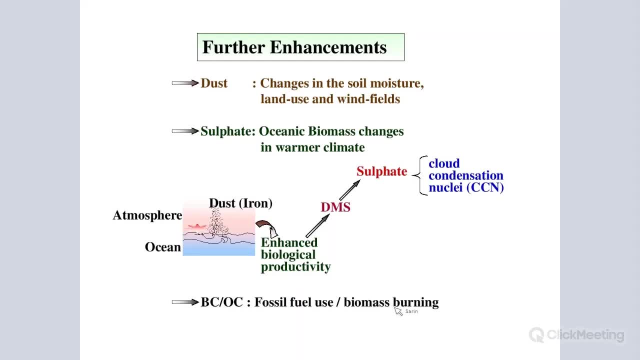 of the black carbon, organic carbon is coming, And the forest fires, biomass burning, agriculture waste residue, these are all adding to the black carbon and organic carbon in the atmosphere, So which I will deal separately on the carbonation aerosol in the tomorrow's talk. 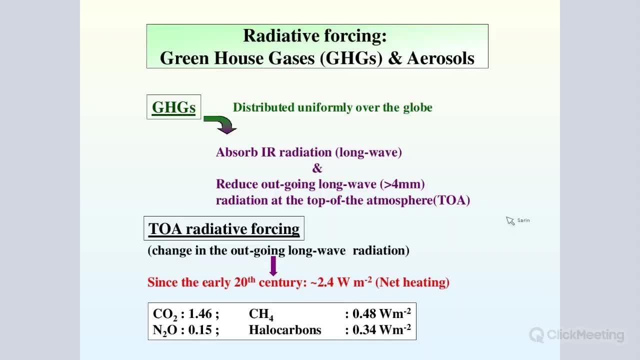 So let us go back to the primary understanding that how does the radiative forcing that means, radiative forcing means the radiation which is coming from the sun, how much is retained by the earth and how much is emitted It is reflected back into the atmosphere so we are able to maintain the balance of 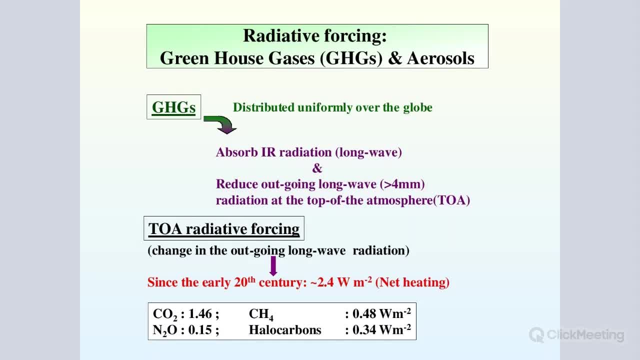 the heat which comes from the sun and how much is going out. So this is where the simple understanding of the greenhouse gases is there: that they are distributed uniformly over the globe. This is something which is very important. That's why the global warming by the greenhouse gases is becoming important, or it has become. 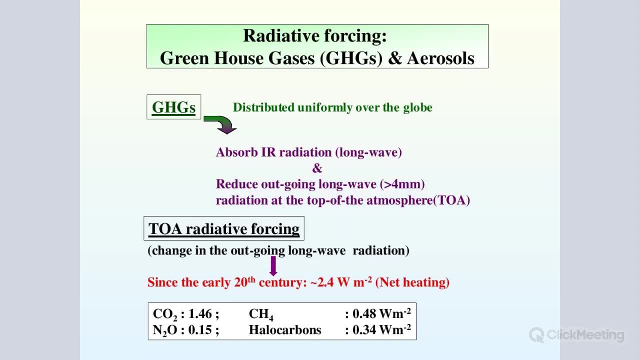 important in the atmosphere In the recent years and people have understood this- that what are the differences in the northern hemisphere versus southern hemisphere? So those are the issues which are important, but we will not get into too much detail because the greenhouse gases and the radiative forcing from greenhouse gases is well understood in. 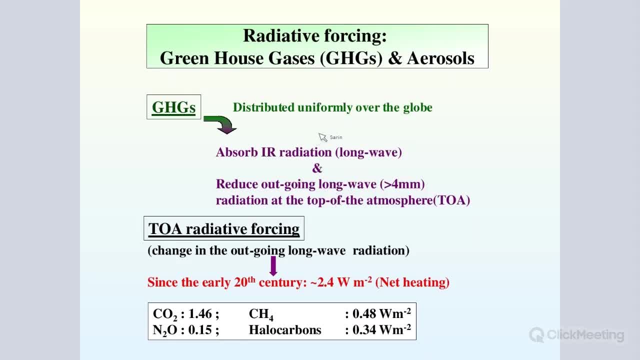 the present day context. So this is, and primarily because they absorb the IR radiation, long wave radiation, and they reflect the outgoing gas. They have the radiation, long wave radiation and then also they have the radiation at the top of the atmosphere. 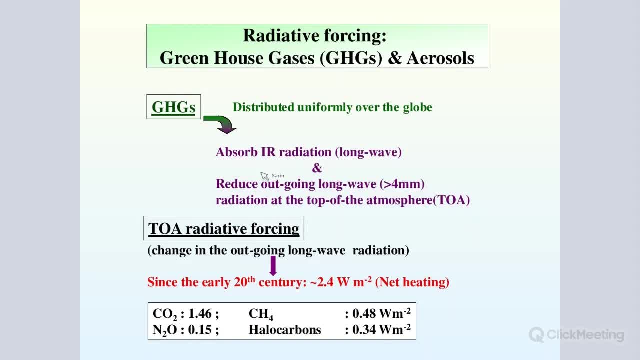 So this is something which is very important- that how the greenhouse gases are maintaining the heat budget in the earth. So in terms of the radiative forcing which is changes in the long wave radiation, incoming and outgoing radiation, So since the early 20th century, which we have now been understanding for the long time. 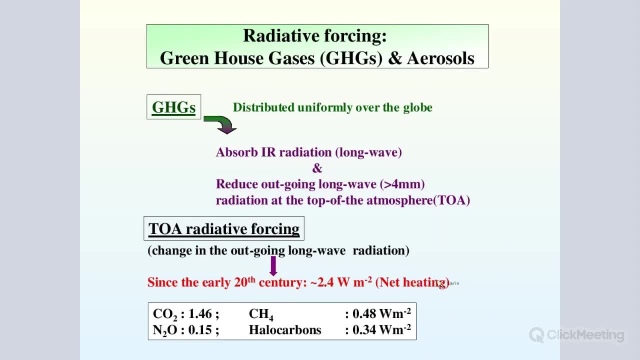 there is a net heating of the order of 2.4 watt meter square. That means whatever heat which is coming from the sun and what is escaping out. there is a difference of 2.4 or 2.5 watt meter square. 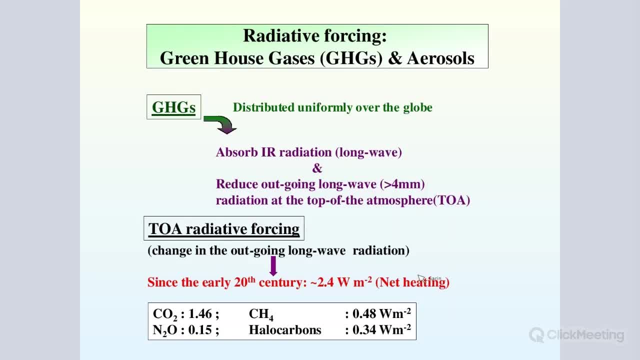 That means we are retaining that much heat in the earth's atmosphere, And this is what is important. This is very important, known as the global warming, which is important in the in the present day context of climate change, as well as the the global warming, and which are integrated. so most of this it comes from the. 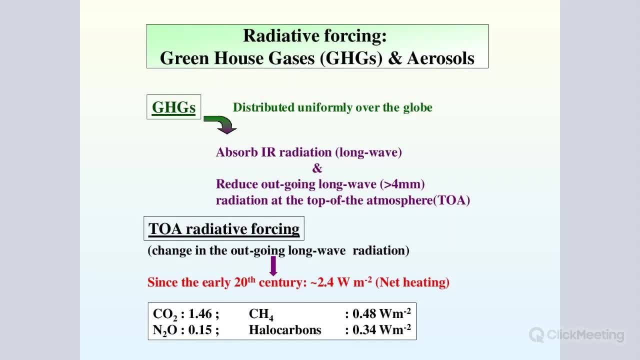 carbon dioxide. all of you have understood that the carbon dioxide is being increasing in the atmosphere from the industrial time, and how so. this is the one of the the most significant greenhouse gas which is adding into the atmosphere and we are having the the maximum the warming is due to. 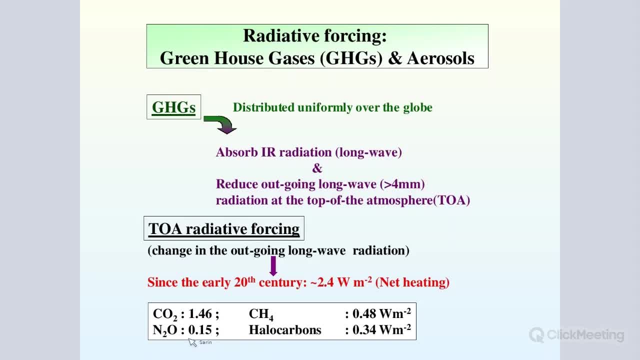 the carbon dioxide, then comes the methane, and then we have the n2o and the other hello carbons. these are all added together. if you see these numbers, they all add up to 2.4 watt meter square. so this is a well understood concept that the that the greenhouse gases are are heating up the atmosphere. 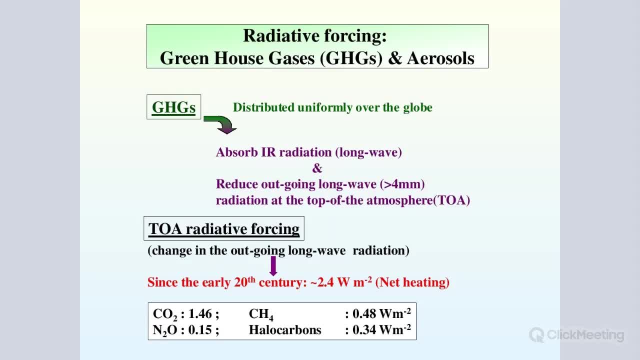 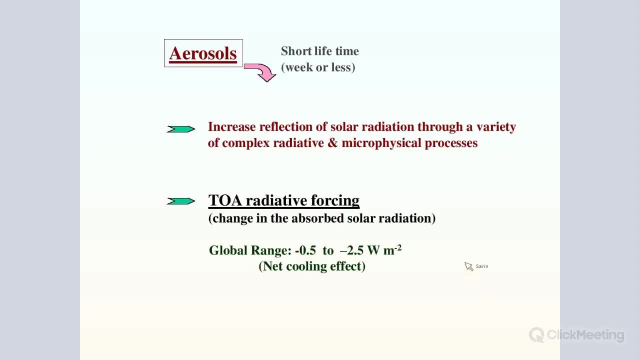 so i will not go into too much details about these things because this is not the primary focus of our today's understanding. so what is important now is the aerosols now, compared to the, to the gases, or compared to the well-mixed greenhouse gases, aerosols have the short lifetime. it is of the order of week. 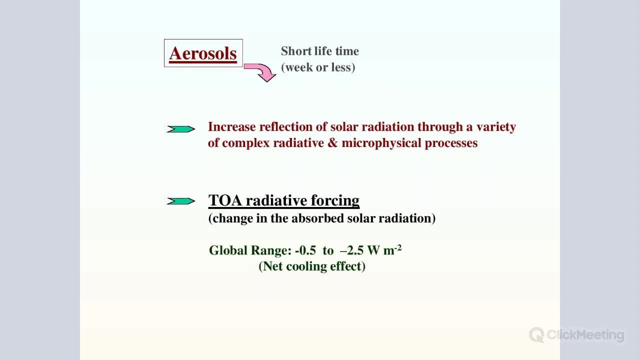 or even less. that means three to four days, because they are. they are removed from the atmosphere very fast, but they they increase the reflection of solar radiation through a variety of of of reasons. I am sorry for the interruption. we'll we'll continue on on this. so these the, the aerosol. 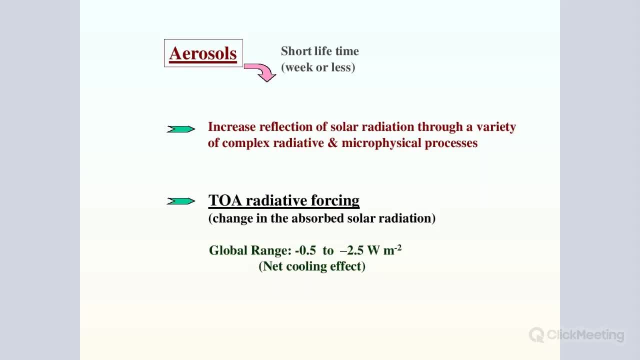 understanding is something which is very important: how it is going to interact with the solar radiation, and something which we we must see that the, how these are, these are are are responsible for the radiative forcing on the top of the atmosphere. so the changes in the in the 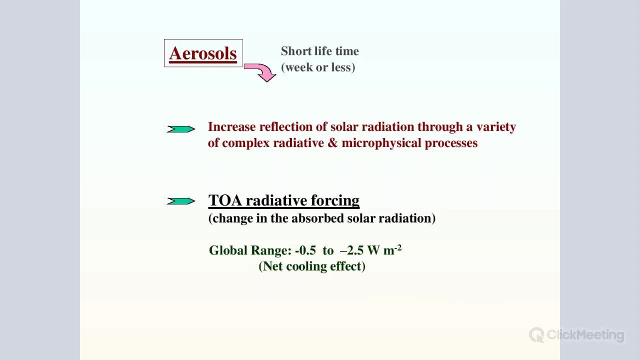 solar radiation and the. if you see the global range, global range is of the order of minus 0.5 to minus 2.5 watt per meter square. now, this is something which is very important. this is the, the present day understanding. so that means, in contrast to the, to the, 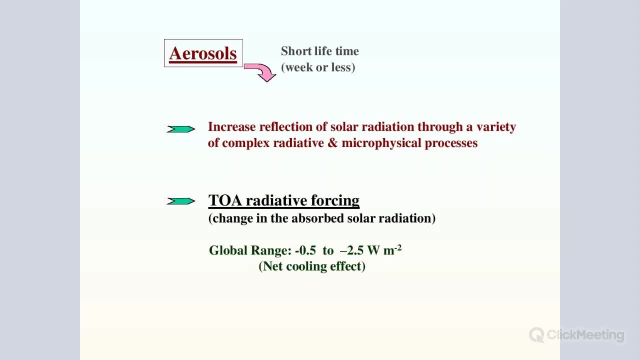 greenhouse gases we are, we are having the net cooling effect due to the aerosol. this is a very simple minded approach which we have to have to further understand, that how this aerosols are having a cooling effect compared to the, to the warming potential of the of, of of the greenhouse. 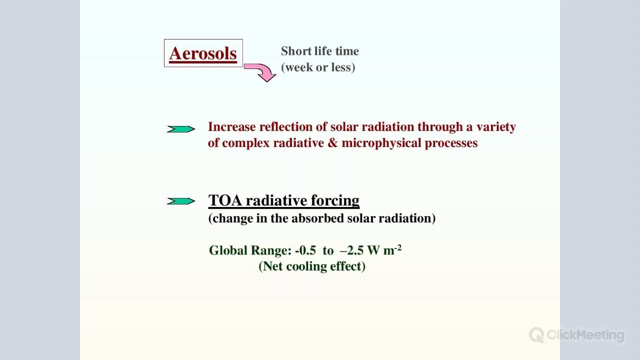 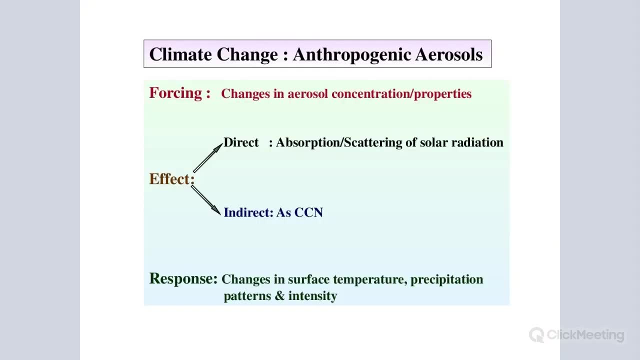 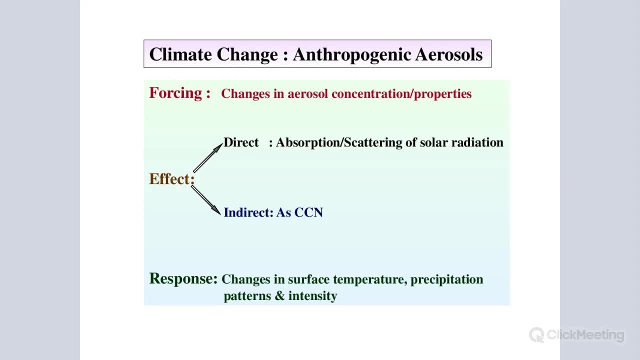 important. so if the forcing is is primarily because of the concentration and the properties of the aerosol, so and and the effect is is seen in the two ways. so this is something which i will try to explain in this and that is the purpose of this uh. 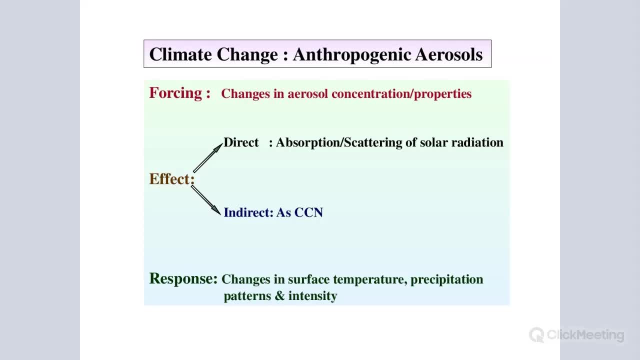 this particular understanding that how are the? the direct effects of aerosols are important and how are the? are the indirect effects of the aerosols are important, as a cloud condensation nuclei, which you, which you see here, and also the absorption and scattering of the solar radiation. 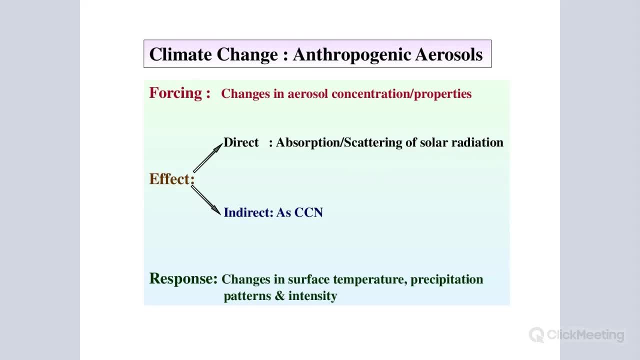 which is considered as the direct effect. so i will try to explain this, uh, this basic concept, in uh, in uh, in this particular context of the climate change uh and largely due to the anthropogenic aerosol. so, as i said, that the lifetime of the of the aerosols is very small, so this we have to keep. 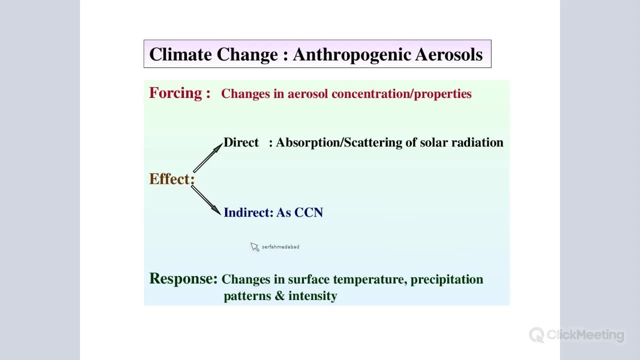 in, uh, in, uh in the mind. so, and the response of this? uh, the climate change. how do we see that? the climate change, how the response is there? so this will be change in the, in the surface temperature and then precipitation, uh pattern and the intensity of the precipitation. this is that the 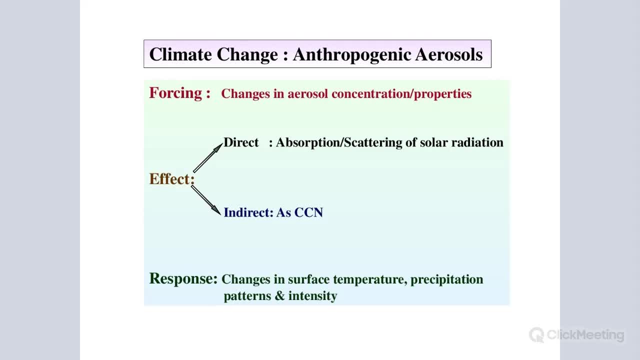 are the response which you can see: whether the climate is changed, because it's a very, very important that the that. how do we know what is the climate change? climate changes is nothing. it has to be seen in terms of the response. so response has to be seen. whether 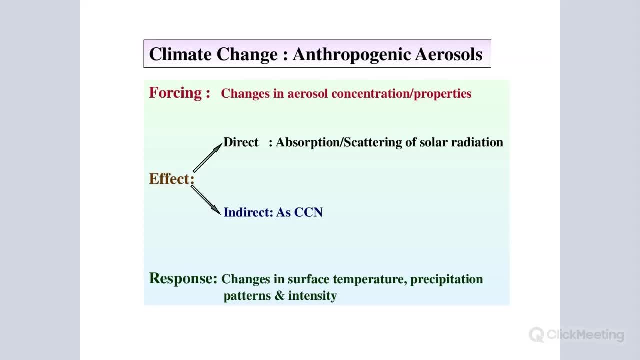 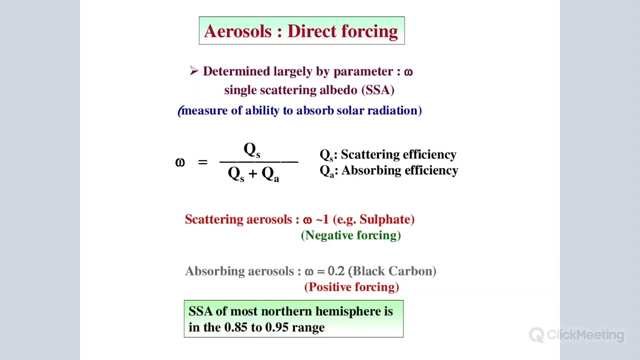 there are going to be changes in surface temperature and the and the precipitation- rainfall- and the intensity. so this is so now the simple understanding: uh is uh. this implies that the, the single which we, we use in the, in the atmospheric chemistry, and that is the ability to absorb the solar 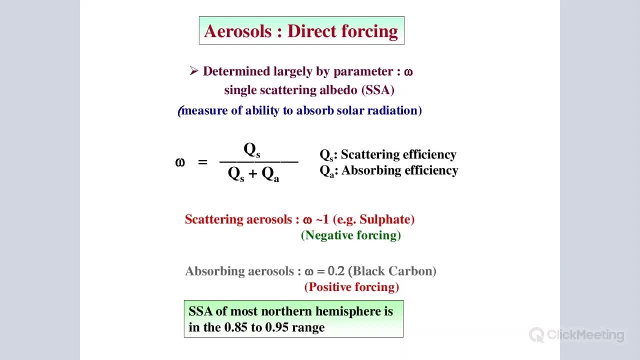 importance and the impact of the aerosol. so So omega is nothing but the ratio of scattering efficiency of the aerosol and some of the albedo scattering efficiency and the scattering efficiency. So this is a simple parameter, which we call as the single scattering albedo, and that determines 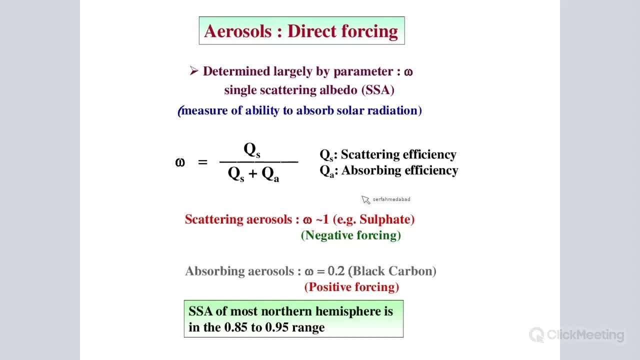 how the aerosols are directly interacting with the atmosphere. So scattering aerosols- the one example which I have given- is as a major impact of the climate or the atmosphere as a negative forcing. that means it is cooling the atmosphere and the omega for the sulphate is very close to 1.. 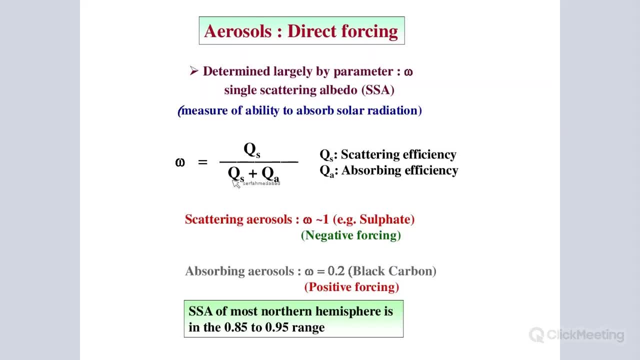 So when the both scattering and the sum of the absorbing and scattering efficiency is equal to 1, that means that particular constituent of the atmosphere is having a negative forcing. that means it is going to cool down, And we all know that sulphate is the constituent which has the cooling effect in the atmosphere. 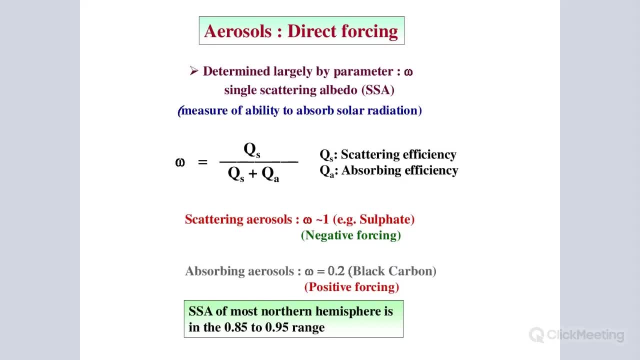 That's why people are trying to do some engineering aspect, that we should add more sulphate in the atmosphere, But that's a different aspect I will not get into much. The absorbing aerosol- and one of the most common examples- is the most important constituent. 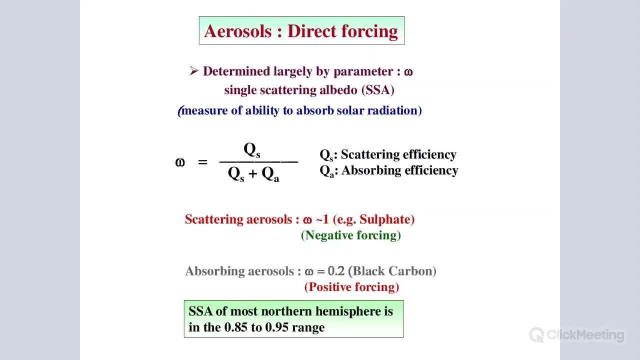 phase in the atmosphere and we have been debating on this. So the first one is the direct forcing from the sulphate, But most of the single scattering in the atmosphere is very close to 0.95 range, So that means 0.8 to 5.9.. So that means the single scattering is very close to 0.95 range. So that means the single scattering is very close to 0.8 to 5.9.. That means the most of the aerosols in the Northern Hemisphere are close to omega value. 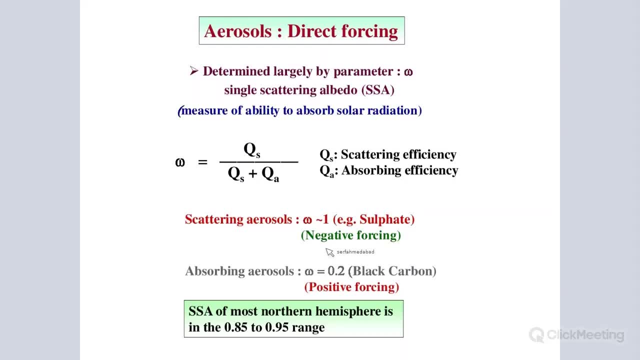 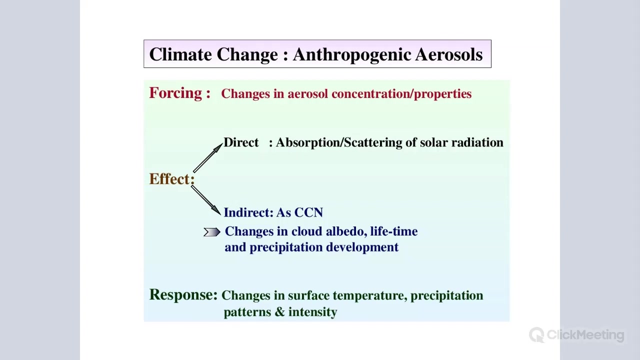 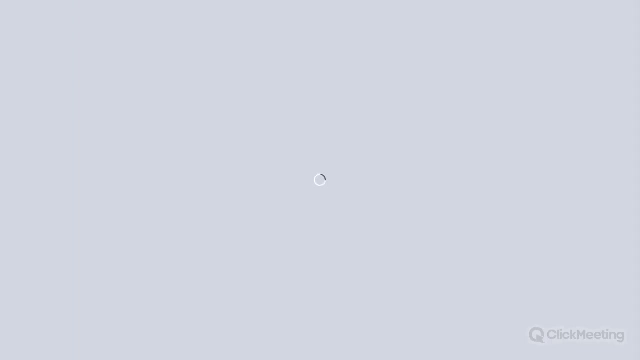 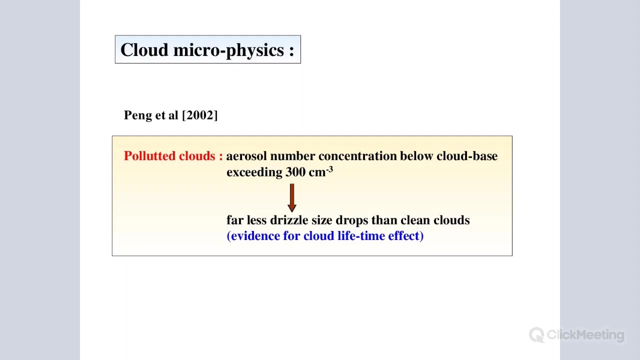 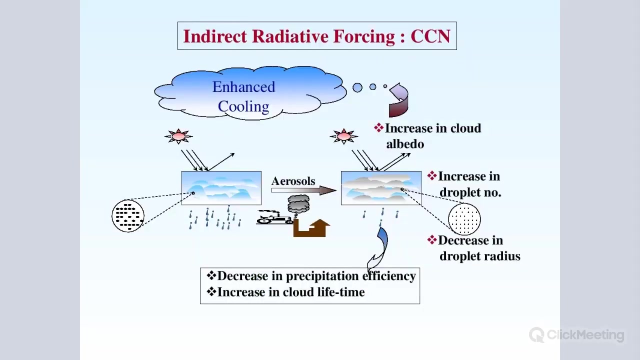 of 1.. So that means we will have a you, you, you, So. So let us try to understand the indirect radiative forcing of aerosol, or what we also refer as the cloud condensation nuclei. So I will try to explain this in a simple concept: that we have a cloud, which is very 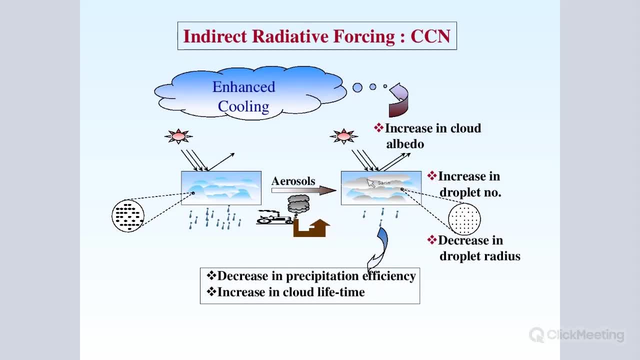 clean and which is not impregnated with aerosol, which you see on the right-hand side. So there is a simple understanding that these have the high precipitation efficiency. they have the large droplets because large droplets are very easy to condense together and you. 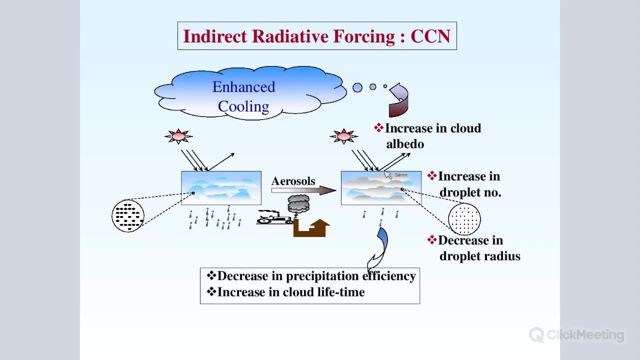 can see the precipitation efficiency compared to the dirty clouds or the clouds which are impregnated with the aerosols, as finally decrease. So this is mainly because of the increase in the droplet number, because once you add the anthropogenic aerosols or the aerosol constituents into the cloud, 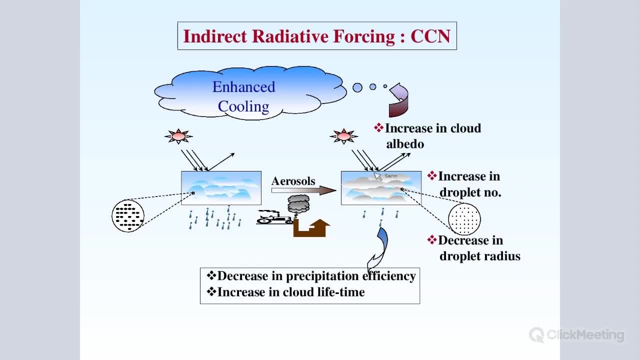 It enhances the number density of the clouds, which you can see the comparison in a conceptual way. So there is an increase in the droplet number and there is a decrease in the droplet radius. So that means you produce very fine drops and you increase the numbers. 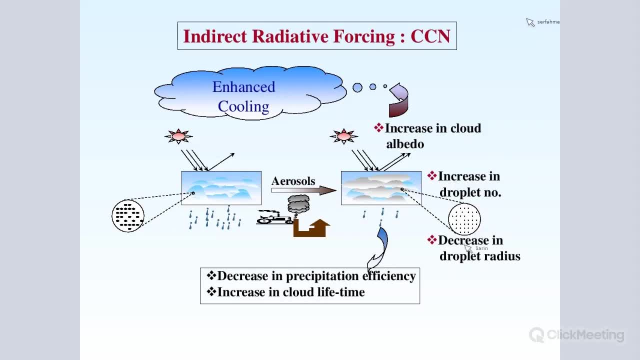 So number density increases, but the drop size or drop the radius decreases compared to this and compared. So this is a simple understanding And because of this there is a decrease in the precipitation efficiency of the clouds, because you are producing very fine droplets which are not easy to condense. 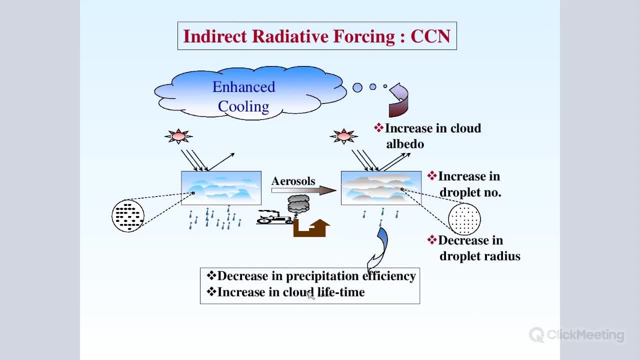 That's why the cloud efficiency decreases and this also has an increase in the cloud lifetime, So lifetime of the cloud will be much longer compared to this particular clean clouds, which has a very high precipitation efficiency, as well as the larger, So this is a very natural scenario. 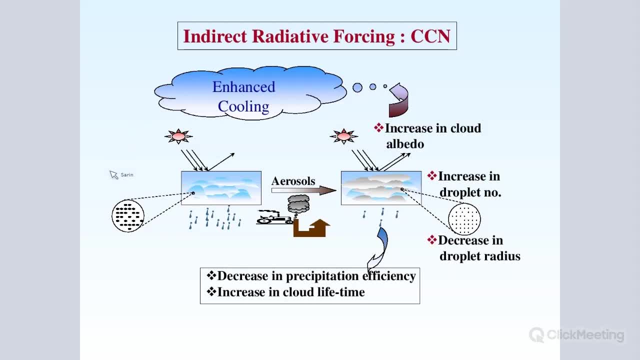 Thank you. So this is a simple example. This is a video which we understand in the simple system, But this is what we are trying to understand: What happens when the anthropogenic aerosols are being added to the cloud system. So you are going to decrease the precipitation efficiency by a simple understanding of the 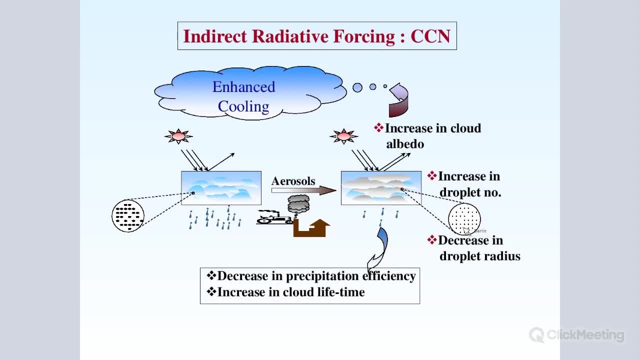 increase in the droplet number and the droplet radius. So this will have the final impact on the cloud albedo, because you are, you are now making a very fine cloud, so this will have the enhanced cooling. so this is the the simple way to understand the uh, the uh, the indirect forcing uh, due to the 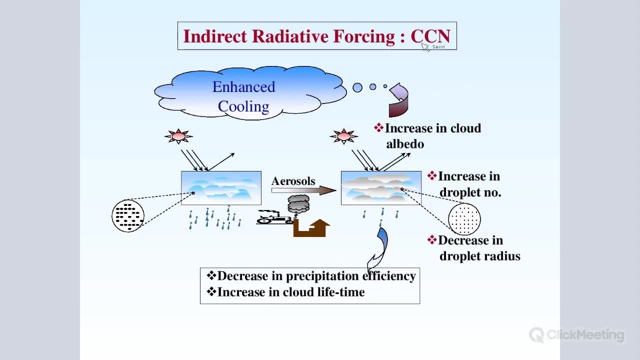 to the aerosols and this is something which is important- that the, how, the, some of the uh, the, the constituents or the aerosol constituents, are that the acting as a cloud condensation nuclei. so ccn stands for the cloud condensation nuclei and this is considered the, the indirect effect. this is a 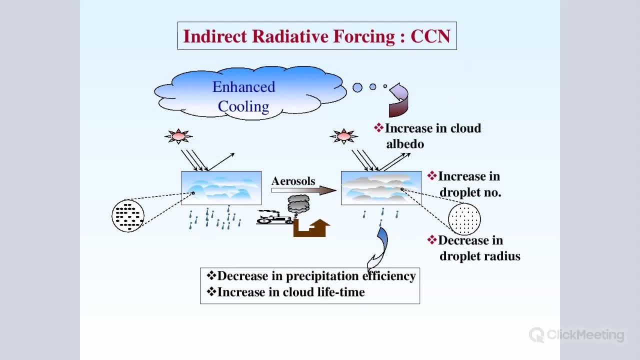 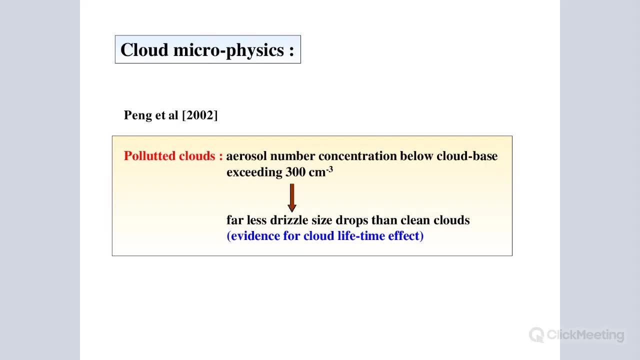 very simple understanding, conceptual understanding, which is, uh, which is important, okay, so so now there are have been some experiments, there has been some, uh, some way to understand whether this is really true or not. so there has been some studies based on the, on polluted clouds, where the 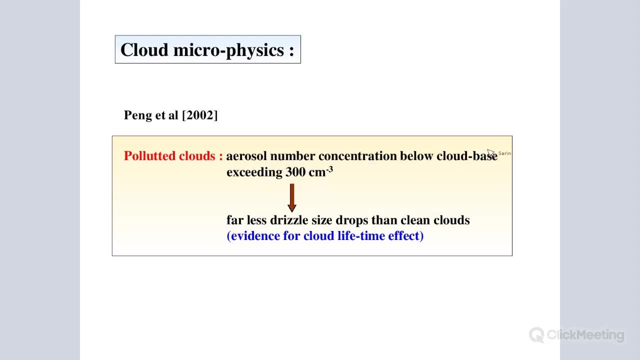 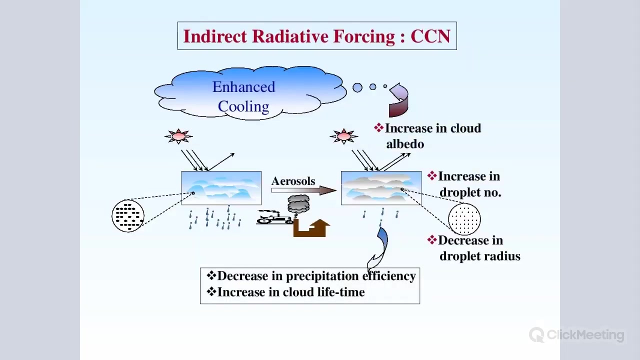 uh if the aerosol number concentration below the cloud base it exceeds the 300 per centimeter cube. so there has been a very far less decrease in the in the, you know, in the drizzle size drops uh that compared to the clean cloud. so people have observed this uh, this kind of uh issue which i i tried to explain in the previous. 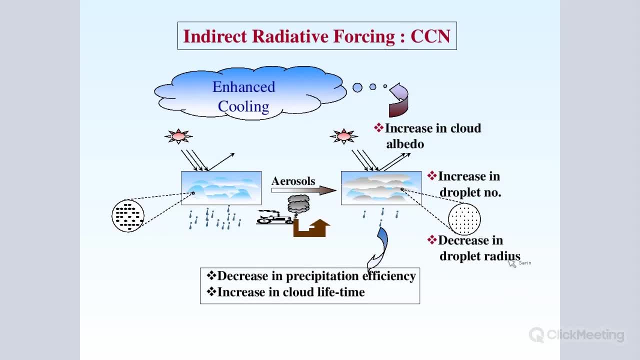 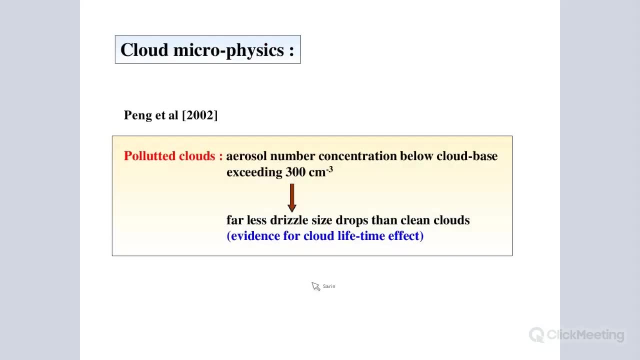 one that the, how, the, the droplet size decreases and the and the density of number, density of the results increases. so this has been observed in some of the, some of the observations, and and people have tried to uh show that the uh, that is, that there is a evidence for the cloud lifetime effect. 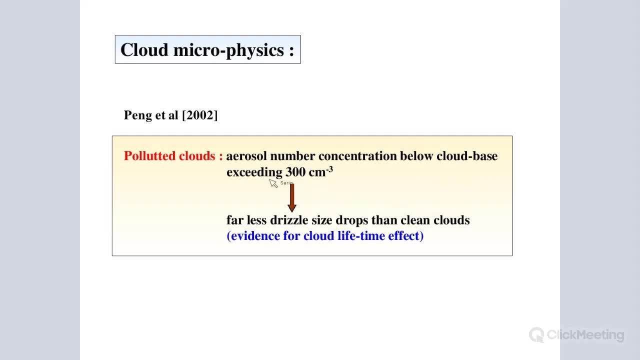 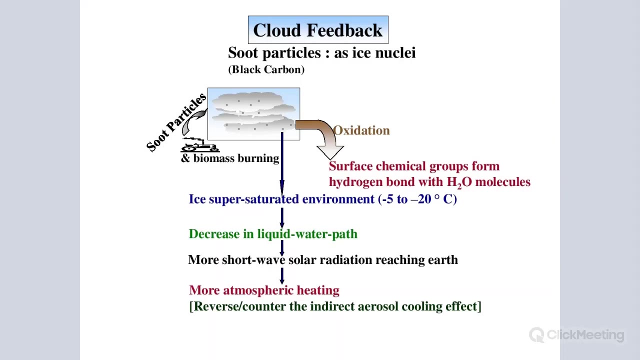 so, depending on the, on the, on the, the number of parasols below the cloud base, so so, so the understanding of the basic concept is: is is being understood in, uh, in a, in based on the observations also. okay, so now the other aspect is that the, the climate system always has a feedback because we, we 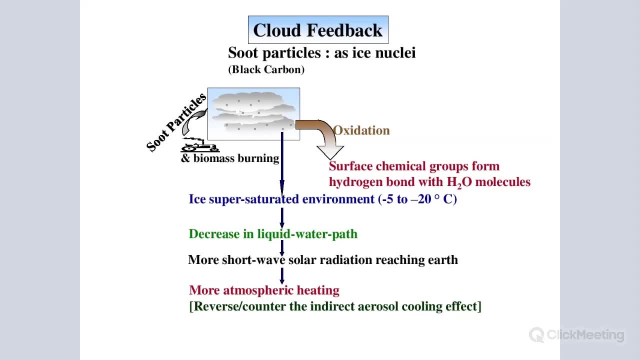 cannot have a one-way interaction because the climate system is not a one-way interaction because there is always feedback. so now the i try to uh so far, uh uh, address that the uh. we have the global uh warming due to the greenhouse gases and we have a general understanding that the aerosols are. 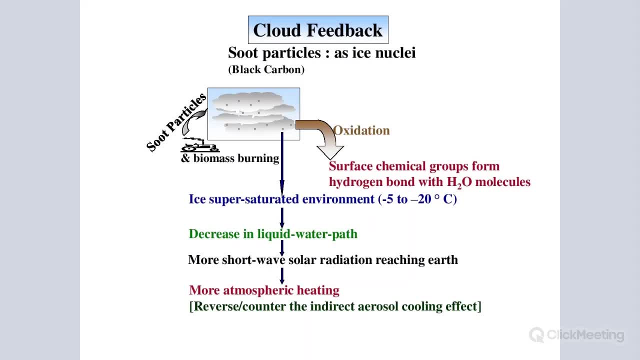 doing the cooling effect in the atmosphere. this can be regional and this can be slightly on a on a larger spatial scale, but this cannot be considered as the as a global phenomena. but nevertheless, the that the overall, the aerosols are having a cooling effect and the and the greenhouse gases are having 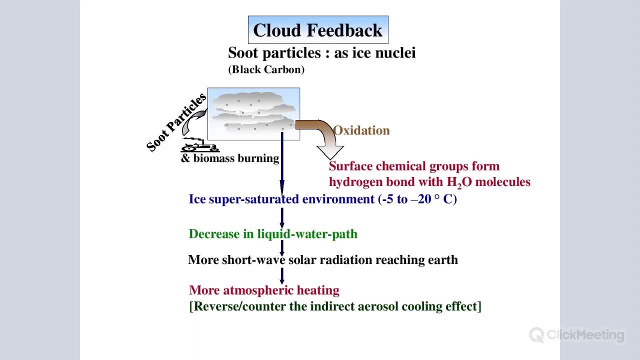 the warming effect. so this is a simple understanding so far I have tried to convey to all of you. so now, but among the aerosols also there is a cloud feedback understanding that the how the some of the aerosols can act as a, also the heating effect, which is contrary to what I try to explain. 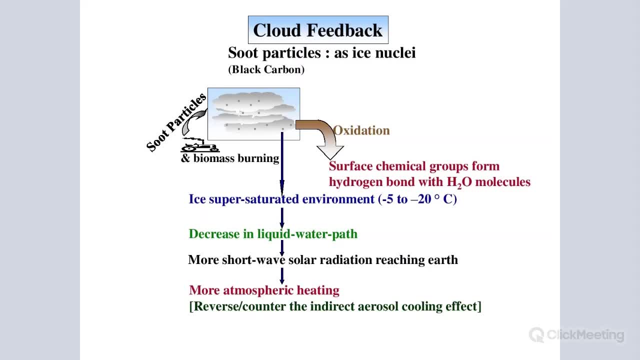 that the direct effect of aerosols and the indirect effect of aerosol. so now, if you take the soot particles of the black carbon and they are considered at the ice nuclei because in the, in the supercooled clouds, at minus 5 to minus 20, minus 20 degrees centigrade, in the in the 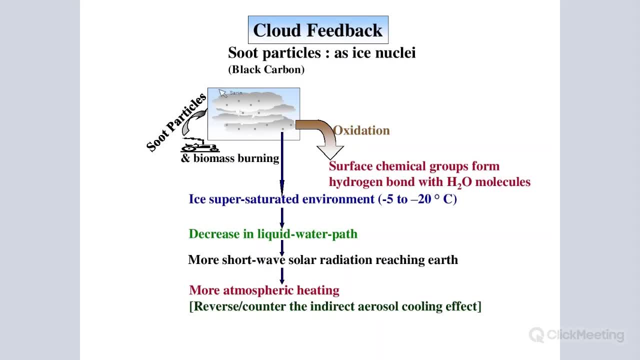 in the high latitude regions. so if we have the soot particles which are which are interacting with the cloud from the biomass burning and fossil fuel emissions, so after some time there is oxidation of these constituents and because of the oxidation, the surface chemical groups which are there in 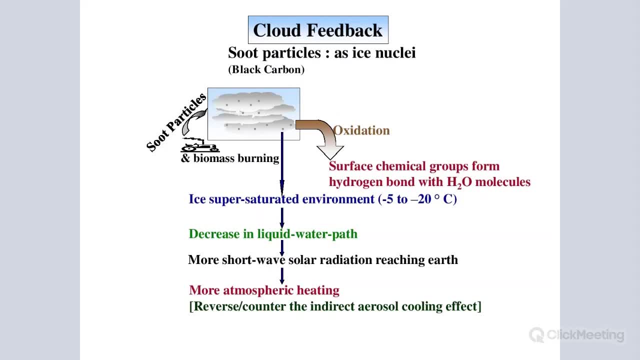 soot particles, because soot particles is a very composite particle, contains the hydrocarbons and contains the other important chemical constituents. so these surface chemical groups which are there in the soot particle, these form the hydrogen bond with the water molecules, because cloud is nothing but the water contained. so it the all. the hydrogen bonding occurs because of the, of the, of the water. 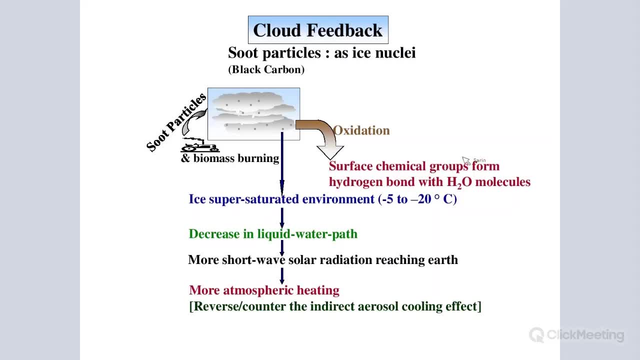 which are present now, if, if these food particles are interacting with the and with the water molecules, with the hydrogen bond. so what is going to have that? in the ice of the, you know it in the eye- super saturated environment, we are going to have the decrease in the liquid. 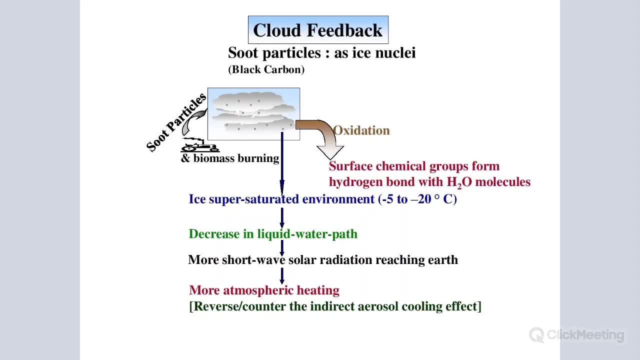 water parts. this is something which is very important. that means you, you are, you are taking away the, the, the water from the, from the clouds, so that will that will decrease the liquid water path, which is very important because the in in general, the, the short wave radiation penetrates. 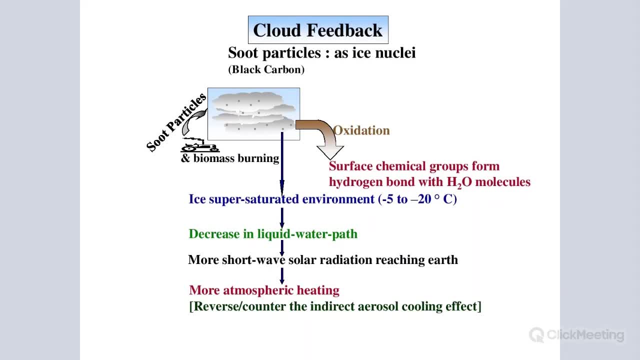 through the liquid, which which has the, which has the uh, the attenuation effect. but if you decrease the liquid water loss, so the, the, the, the, the more short wave radiation will reach the earth. this is a simple understanding in this. so if, if we are removing the water, 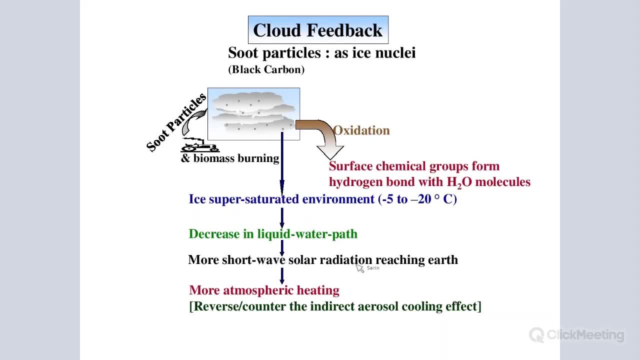 we are, we are, we are allowing more short wave uh the solar radiation uh to to reach the earth surface. so this will have a have a uh, a more uh, you know, heating effect on the, on the atmosphere. so more heating due to this. so this is going to have a counter the uh, the the cooling effect. 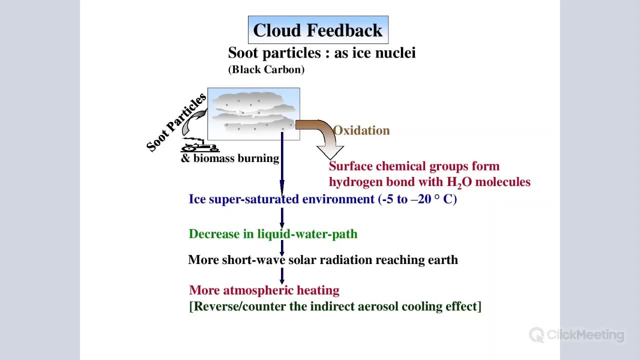 which we have talked about in the in the in the last few minutes of the of the air. so there is a feedback now because of the some of the particles. so instead of now- uh, now- cooling the atmosphere due to anthropogenic aerosol, we are invoking the concept of of heating the atmosphere. 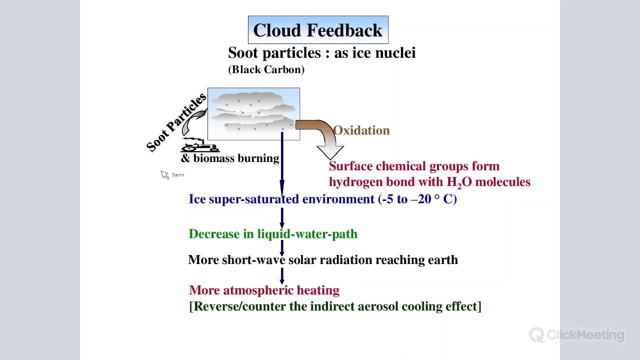 because of the interaction with the clouds and because of the soot particles which are being added into the atmosphere. so this is a, this is another type of understanding which we have to keep in mind, that the, how, the, the feedback mechanisms are are also important in the, in the in the present day. 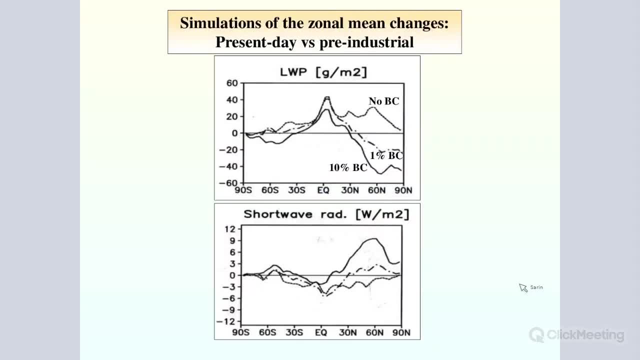 context and in the atmosphere. so there has been some simulation studies which have been done based on the previous concept which i talked about, that people have have seen that the uh, that if you take the liquid water path which i talked about in the previous uh, uh slides, that if there is no bc, 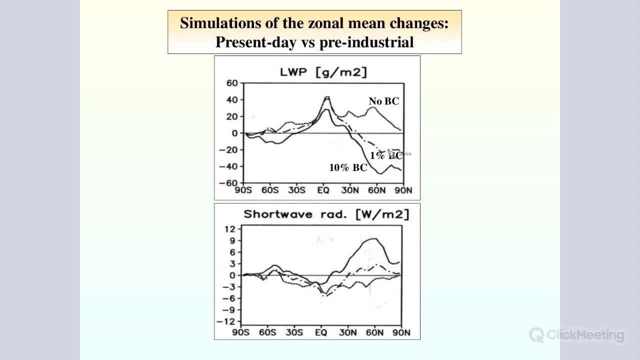 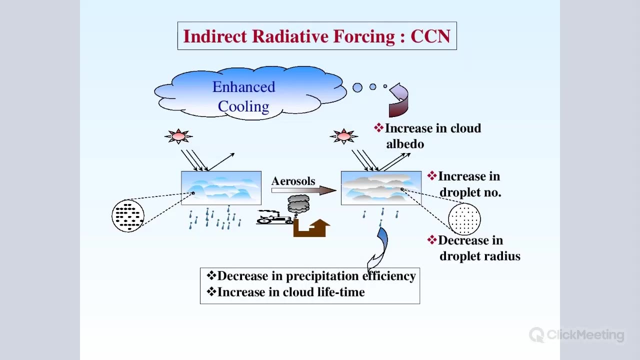 and with the, with the one percent of bc concentration put in the system, and if you have 10 bc concentration in system, and what happens to the liquid water path? so you can see that the liquid water path increases. uh, when, when there is no black carbon, which i explained in this concept. 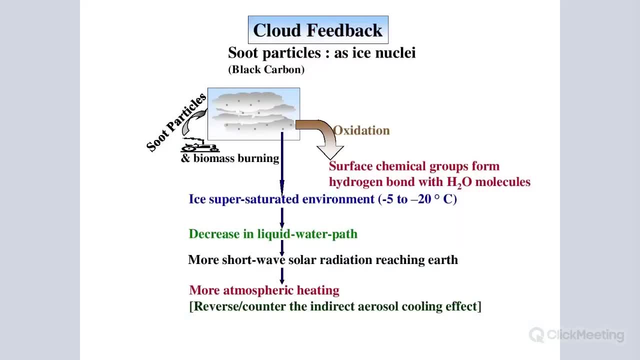 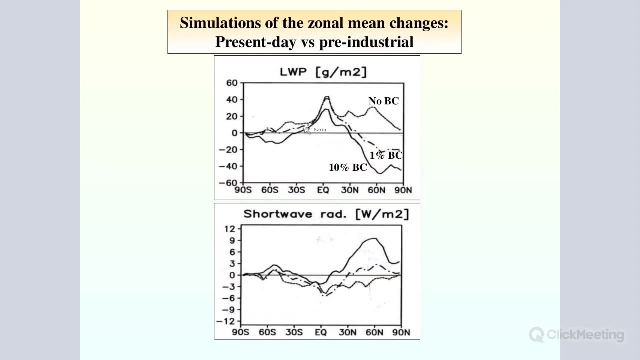 uh in in this concept that the, the hydrogen bonding with the suit particles will uh will will take away all the all the water molecules, so liquid water path will uh will decrease. so this concept is is being uh studied in based on the modeling approach, that if there is no black carbon, 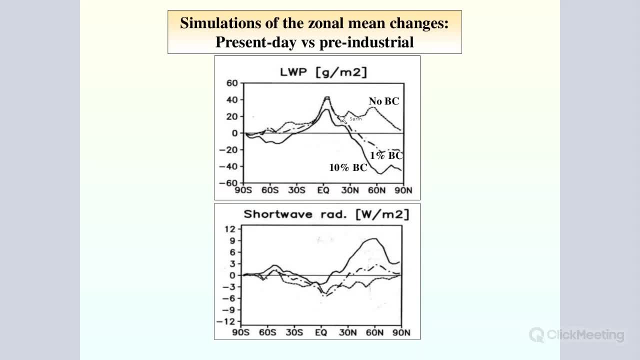 then the liquid water path is is more. and if there is one person, uh, one percent bc, then you have a liquid for water path bc. so if there is no black carbon, then the liquid water path is decreases and if you have 10% BC, there is a further decrease in the liquid water path. 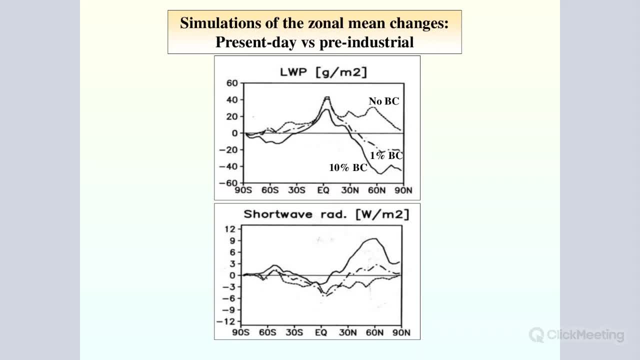 So this is in units of grams per meter square. this is a standard way of doing the simulation, and most of these are important in the northern hemisphere because that's where we have more anthropogenic activities compared to the southern hemisphere. Now, in response to this liquid water path which you have seen in this top picture, what? 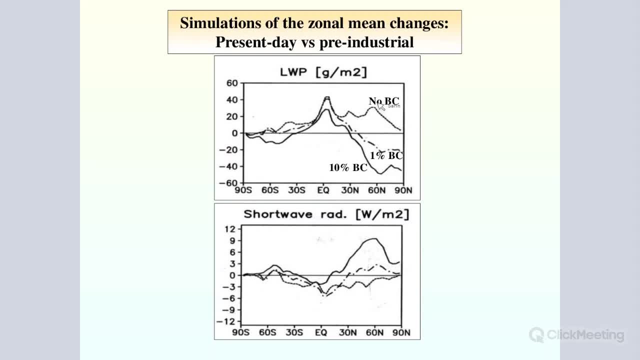 happens to the shortwave radiation. now, If you see that when there was 10% BC, you have more penetration of the shortwave radiation. So this is something which is what the previous cartoon or the conceptual way of understanding was there: that you have more penetration of the shortwave radiation when there is a high 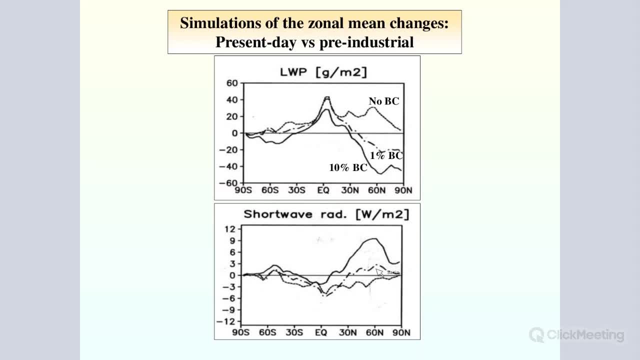 concentration of BC in the atmosphere and when you have the 1% BC, the shortwave penetration is less, And when you have no BC, there is no penetration of the shortwave radiation. That means you have a negative forcing, but in this case you have the positive effect. 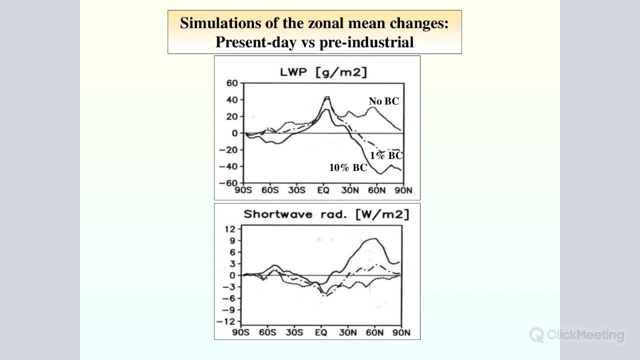 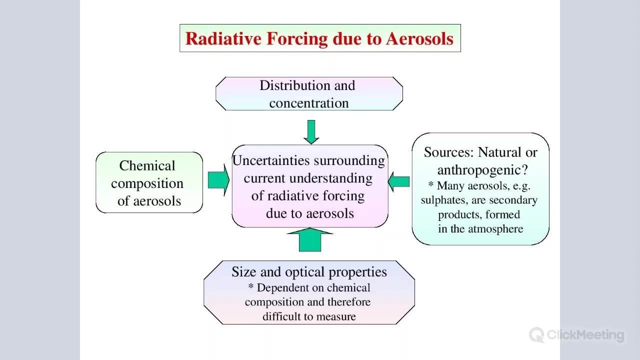 you are allowing more shortwave radiation to come to the earth. So this is a very important way to understand. how does the feedback mechanism as well as the indirect effect of the aerosols is important. So, coming further to the now final understanding, because whatever I said in the introduction, 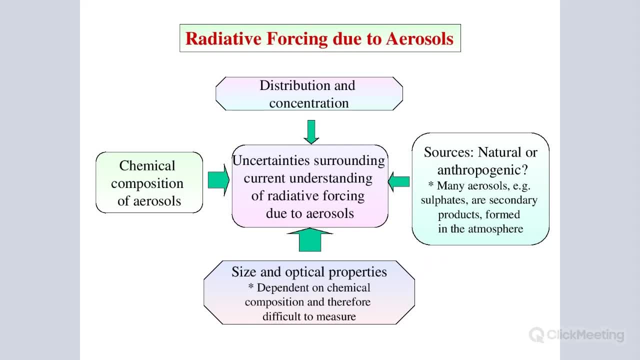 I will be repeating it in the last couple of minutes- that the radiative forcing due to the aerosols. So the important thing is: what are the uncertainties which are surrounding the current understanding of the radiative forcing due to aerosol? The size of this arrow or the thickness of this arrow tells you. the greater the thickness, 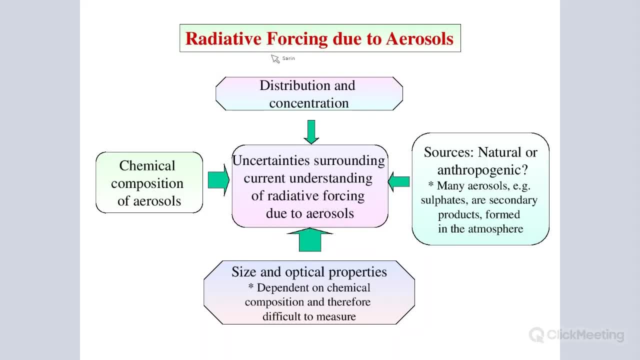 higher is the uncertainty because of that particular one. So let us see the first one. the smallest uncertainty is coming from the distribution and the concentration. That means we have to see the concentration, So let us see the first one. We have to still understand what is the distribution and the concentration of the atmospheric aerosol? 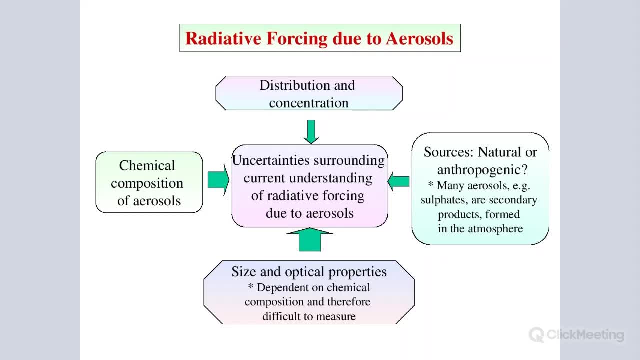 But most of the uncertainty which is coming in our understanding and coming in the way of putting the impact of the aerosols on the climate change is largely because of the size and the optical properties of the aerosol, Because this is something which is very important and that depends on the chemical composition. 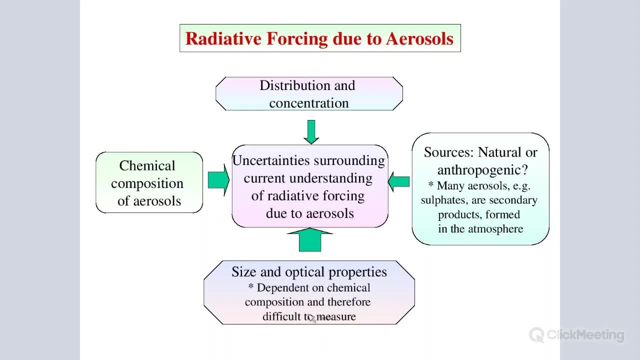 as well as the And, which is more difficult to measure. Then we also have to understand all the uncertainties coming into the picture because in the radiative forcing due to aerosol is largely coming from the aerosols which are natural or anthropogenic And- this is a very important aspect- how the sulfates are the secondary constituents in 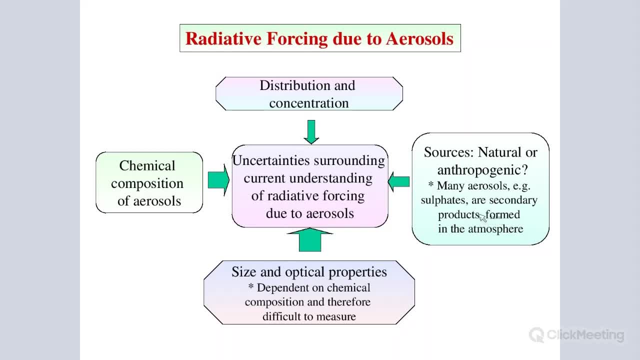 the atmosphere and what are the role of the secondary particles in the atmosphere. So this is a very important aspect. So the uncertainty in our understanding is also due to the sources of natural as well as the anthropogenic- Another major uncertainty, because thickness of this arrow is pointing towards the chemical. 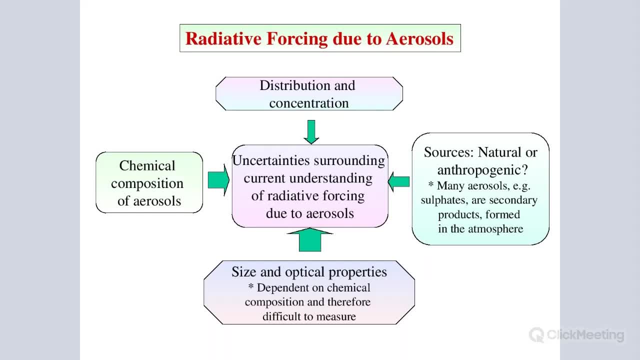 composition of aerosol. Now people are trying to understand the chemical composition of aerosol And, unlike the greenhouse gases, which are well mixed in the atmosphere, inter-hemispheric differences are not large, But aerosols are well mixed in the atmosphere. 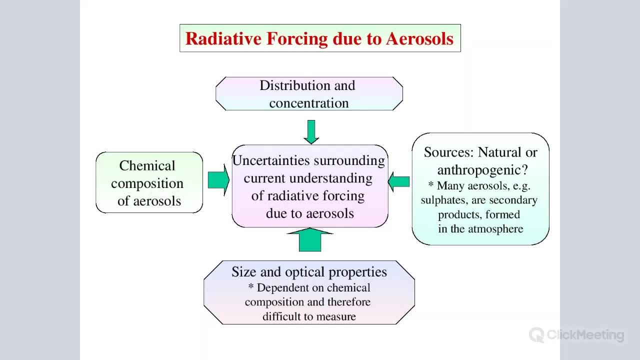 So aerosols are very highly regional, highly localized. So one has to understand the chemical composition of aerosol both on the regional as well as on the spatial scale. So this is an important bottleneck in our understanding of the radiative forcing due to aerosols. 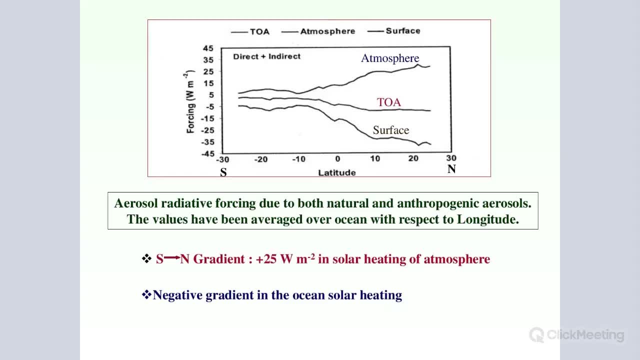 Okay, So let us now try to understand the whatever- or I will try to summarize whatever I have said in the last slides, In the last 20 to 30 minutes, that the aerosol radiative forcing due to both natural and anthropogenic aerosols. 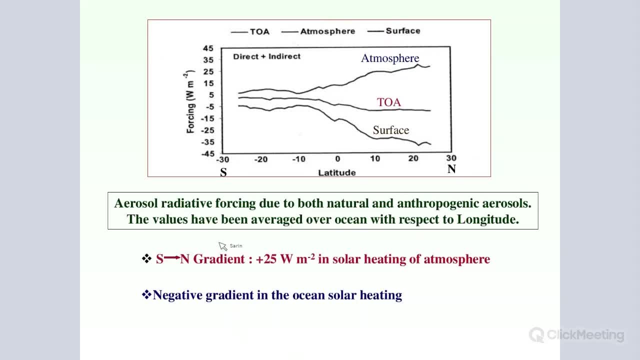 This is what this picture is trying to convey. I will try to explain this. And the values have been averaged over the ocean with respect to the longitude, Of course, you see a latitude distribution of the forcing which is in units of watt per meter square. 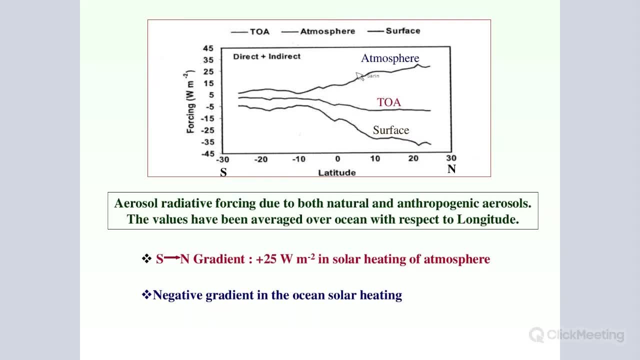 But this is very important to see that how this forcing is there in the atmosphere, top of the atmosphere and at the surface. So this is the what. the message which is coming from this is that the surface has been averaged over the mean with respect to the longitude. 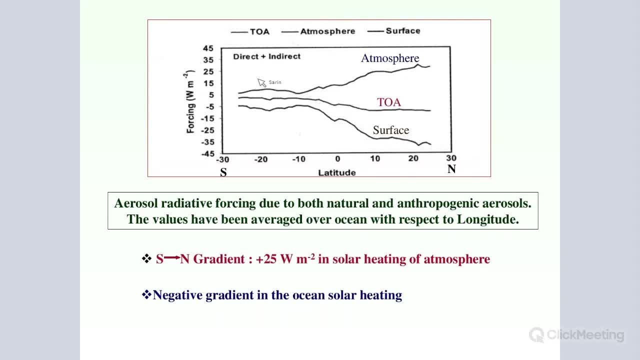 So that means this is the over the oceans, this is a mean has been taken, whereas the atmosphere and the top of the atmosphere. So what you see? a very conspicuous trend. There is a south-north gradient, so if you go from southern hemisphere to northern hemisphere, 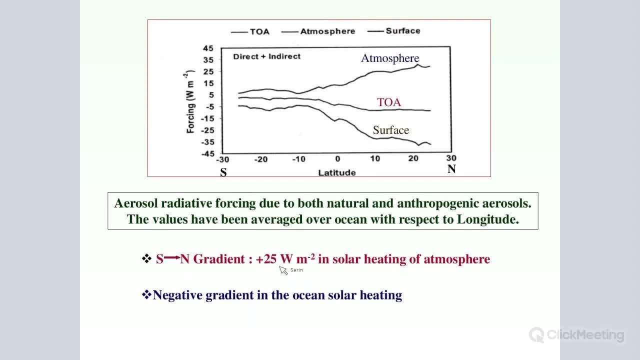 you see a south-north gradient That means almost of the order of minus 25 watt per meter square in the solar radiation. So this is something which is known as the heating of the atmosphere. So and the forcing, which is important. And then you also see a negative gradient in the ocean: solar heating. 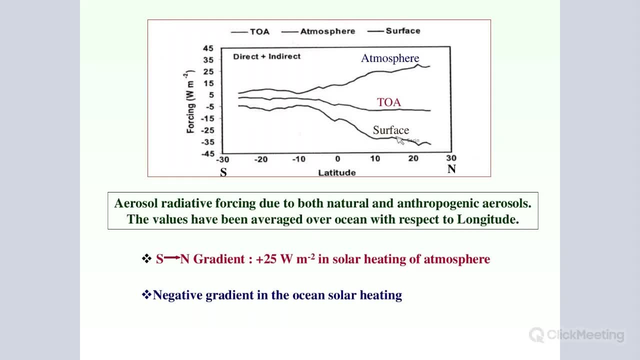 That means this is the surface heating, So you see a negative trend in this. So this is what we have been trying to talk about: that the aerosols have been having a counter impact compared to the greenhouse gases. that the aerosols are having the cooling. 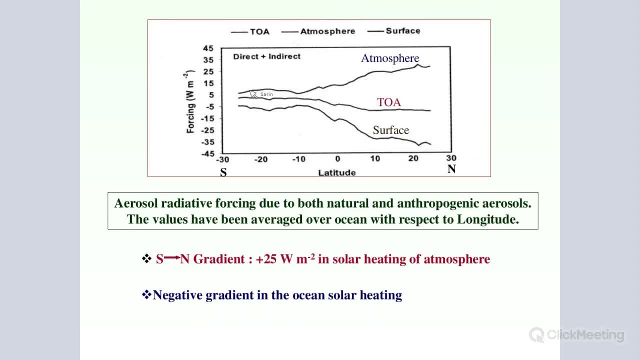 effect. But if you see the top of the atmosphere, there is a net cooling of the order of whatever which I explained in the previous slides, of the order of 5 watt per meter square, But on the on the atmosphere as such is heating, but the surface is cooling as well as the top. 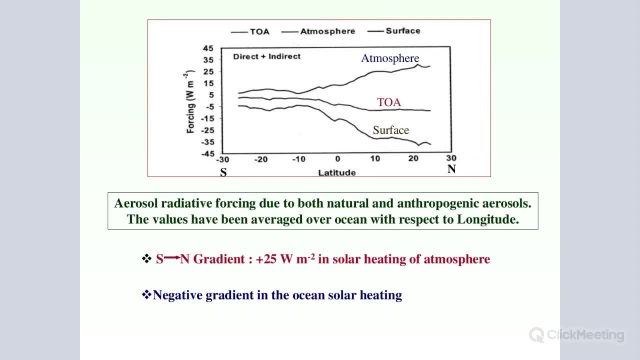 of the atmosphere is cooling. So this is the simple understanding which we have so far about the aerosol. But this is a very elementary and simple understanding so far about the about the anthropogenic aerosols. So these are based on simulations as well as the observations. 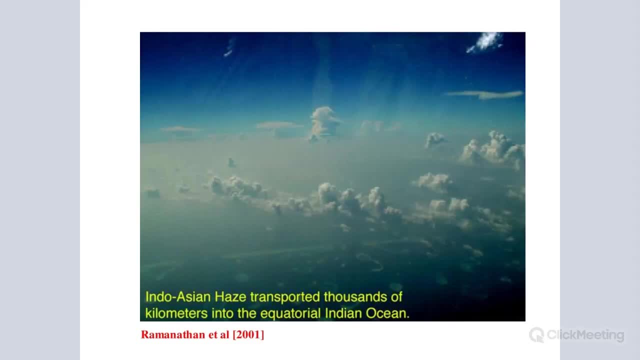 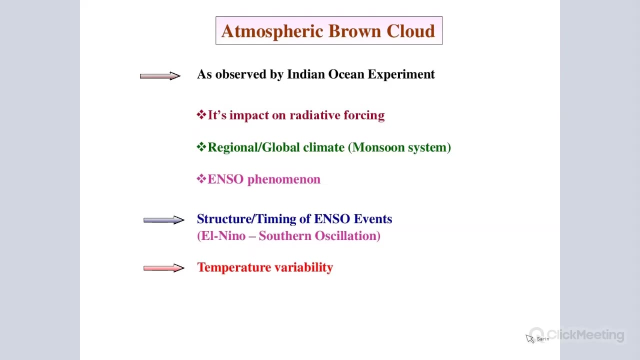 So so, in coming to the to the some of the observations, this is: this is the Indo-Asian Haze transported thousands of kilometers to the equatorial Indian Ocean. This was was mainly was part of the atmospheric the brown cloud program which was there in. 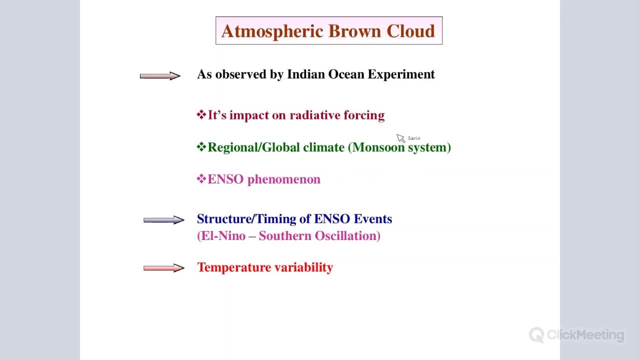 the Indian Ocean experiment and its impact on the, on the radiative forcing and the regional and the And the global climate, how the response is there, how it is there, And then also to understand the ENSO phenomena, which is nothing but the El Nino Southern Oscillation. 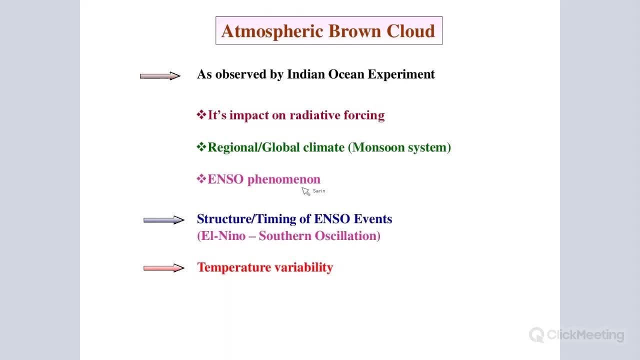 which I will not get into my details right now. So these are the, this was the, this was the basic objective of the atmospheric brown cloud: to understand that the how, the, the, the processes over the, over the ocean or the, the marine atmospheric boundary layer are important. 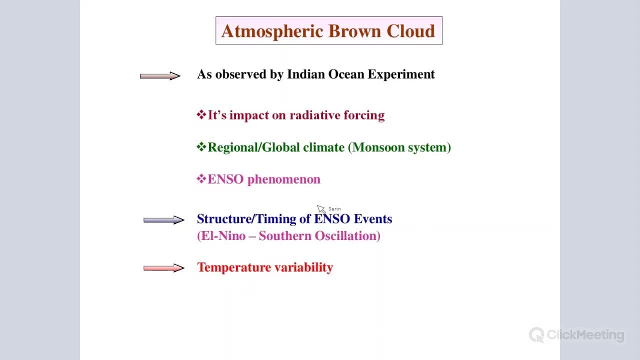 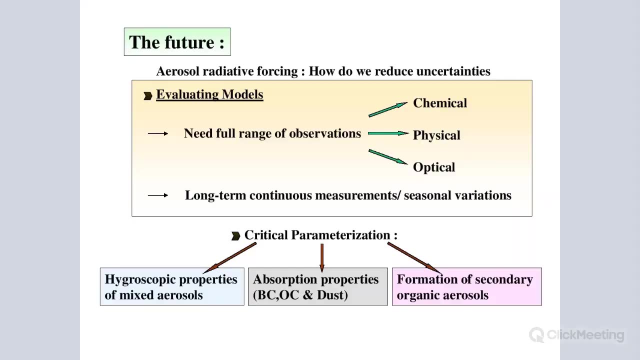 So And also how the, the temperature variability is, is, can be understood in that. So, Coming to the future, how do we are going to understand the our approach in the in the future scenario, Aerosol radiative forcing- How do we reduce the uncertainty which I tried to explain in the in the previous slide? 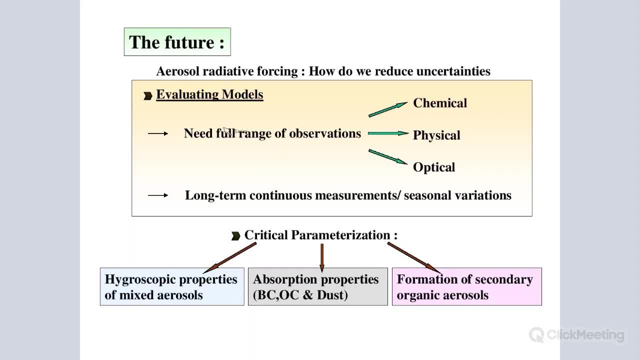 also that the how do we try it So? So we need a full range of observations, and these observations have to be chemical, physical and optical properties of the aerosol. So we must understand the size, composition and the optical properties of the runner. 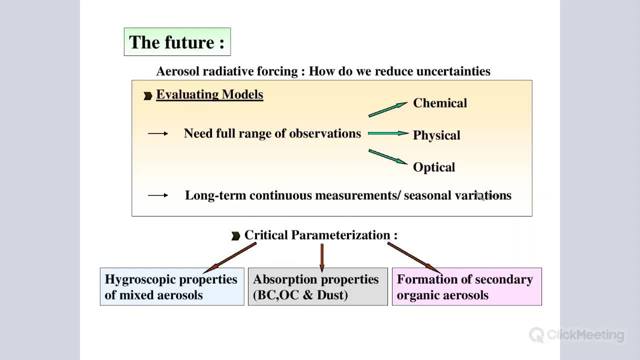 And the long-term continuous measurements and the seasonal variation, which is very important, the estimates which have to be done because unless we know the long-term continuous measurement- because the lifetime of aerosols is very small as well as there are regional variations- 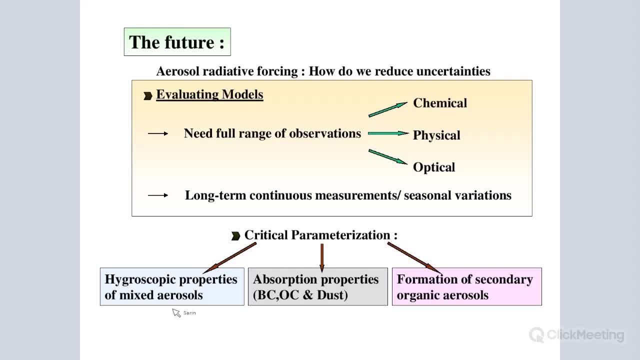 So we have to have the critical parameterization of the hydroscopic properties of the mixed aerosols, because aerosols in the atmosphere are not an individual constituent. The dust is mixed with the black carbon and all the sea salts are mixed with the dust. 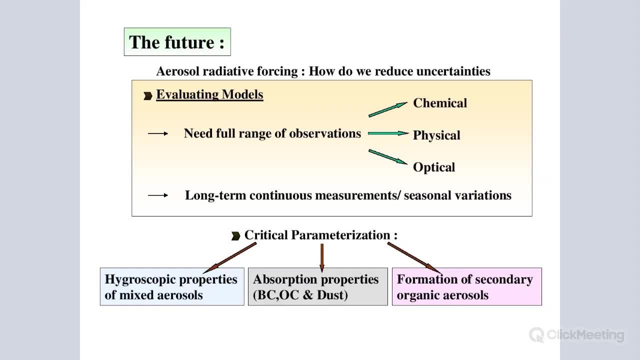 And so we have a very mixed type of aerosols in the atmosphere. So we have to understand the absorption, So we have to understand the absorption properties of mixed aerosol, And these are mainly the black carbon, organic carbon and the dust. 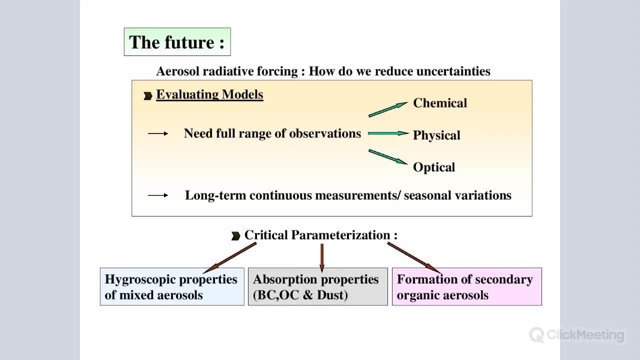 I will in the next two or three talks I will dwell upon the role of black carbon, organic carbon, in the atmosphere. So this was the understanding to see as a basic on the anthropogenic aerosols which are important in the atmospheric radio-diffusing. 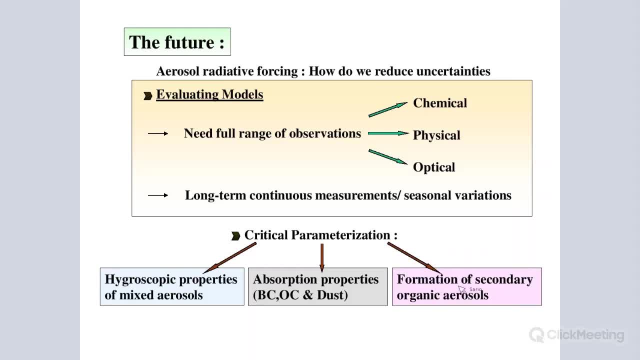 So formation of secondary organic aerosol, This is a big question. We do not have much understanding so far, but this is the most important thing, because secondary aerosols, organic aerosols, are very important in the atmosphere. So this understanding has to be there in our future approach. 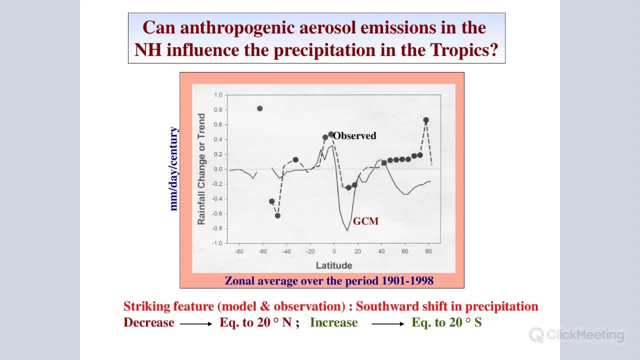 Okay, So there is some concept which has so far evolved that the understanding that the- and this is one of the climate impact or the climate forcing from the anthropogenic aerosols. The question which people ask is that can anthropogenic aerosol emissions in the Northern 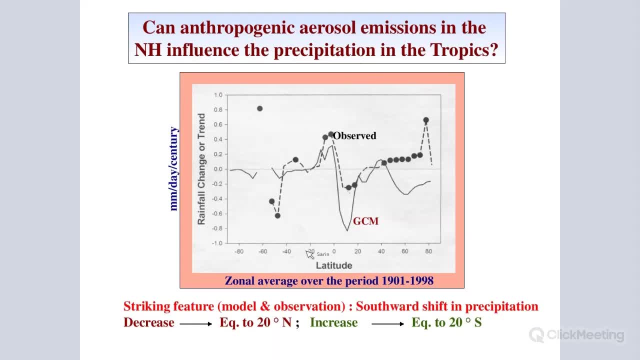 Hemisphere influence, the precipitation in the tropics. So I would like you to focus on this region, because we are talking about the tropics. So you can see, this is the observed phenomena which is shown by the black dots, and this is the global circulation model which is also trying to mimic, except that there is 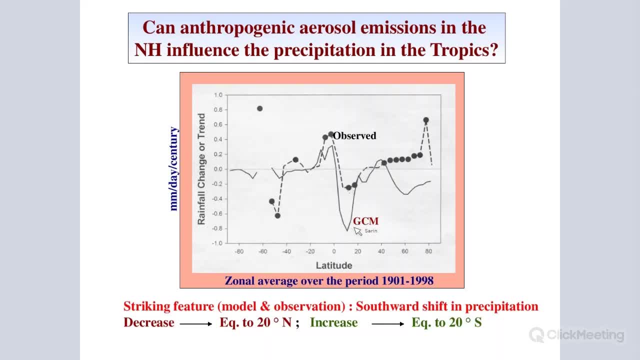 some differences in the observation and the model and the model in the in in the more in the tropical area. but what this particular study or what this particular the message which is trying to get out from this comparison, from long-term observations and the data versus the model? it says that this striking feature in the 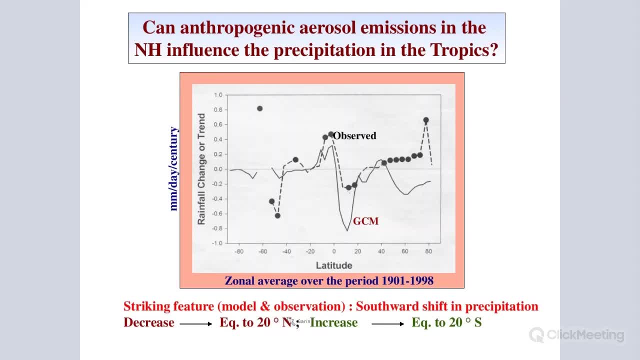 is is important for the in the model and the observation, and there is a southward shift in the precipitation. so if you, if you see that the, the precipitation is is increasing in the, in the million, in the southern, the south of equator, which is what we can see, therapy: this is a decrease in. 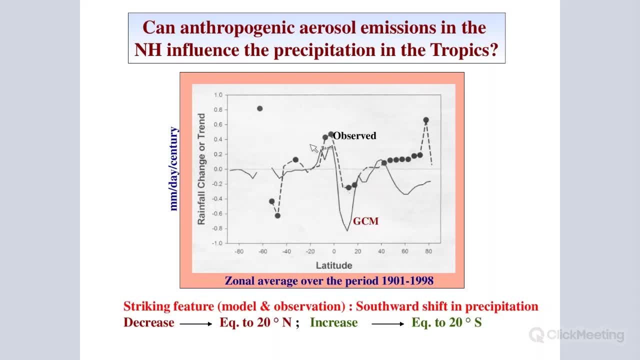 the, in the, in the precipitation. but when you come to the south of the tropical region there is an increase in the precipitation. so the, the re, dark night, equator from 20 degree not to equator. so there, the decrease from the 20 degrees not to the earth, to the left, to the south, one is a total. 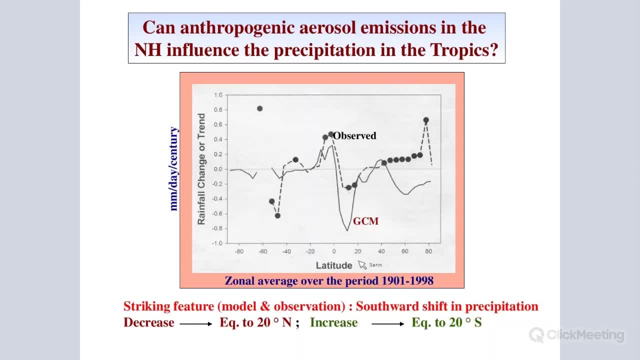 of even as adventure, in which is very good. system control destruction function here lead neither to equator, and there is a increase in the equator to the 20 degree south. so this is a something which is a which is very important that people are trying to understand this. 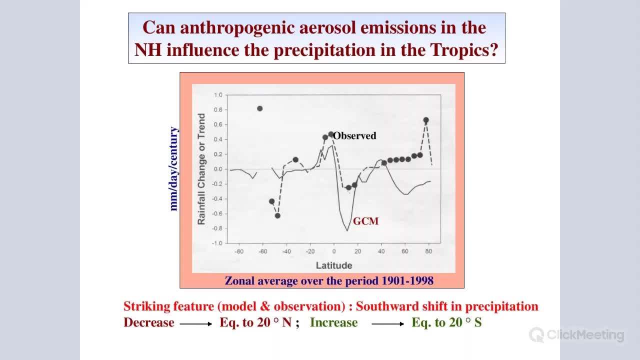 the aspect- and this has a very, a very major implications- that the dust anthropogenic aerosols in the atmosphere are going to influence the precipitation in the tropics. this is something which is we have to understand and there has to be more understanding in in our had to be developed in the in the due course of time. so i will try to come to the 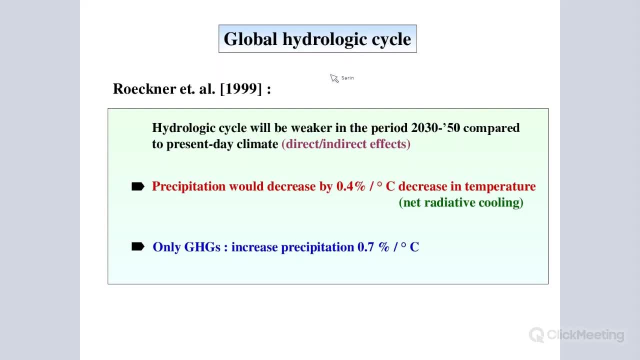 conclusion. so the global hydrological cycle, which is which has been now looked at it, so there are, there are some understanding in this aspect. so people are trying to say that the hydrological or hydrologic cycle will be weaker in the period from 2030 to 2050 compared to the present day. 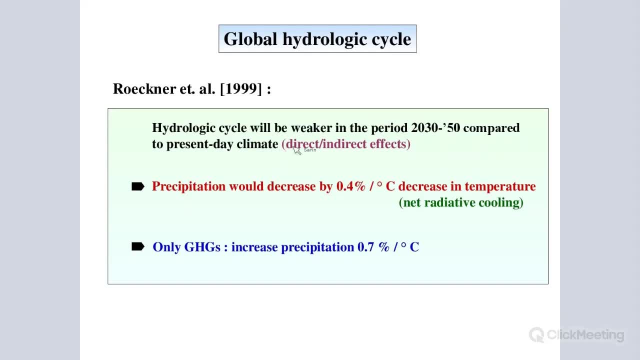 climate. this is a very important conclusion which has come from the study which was done several years ago that the and on the on the global hydrologic cycle, and this has both the direct and the indirect effects of the aerosol which i tried to discuss in the last one hour. 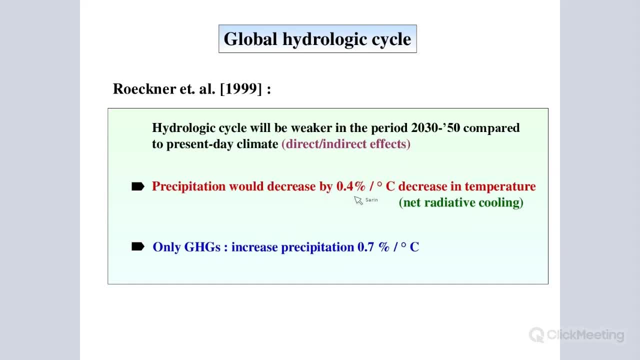 and the a higher air pressure. the air pressure in the air pressure was raised and indeed what it has done is that it has allowed the air pressure to be reduced by 0.7 percent and precipitation would decrease by 0.4 percent per degree centigrade. that mean decrease in the temperature. this will 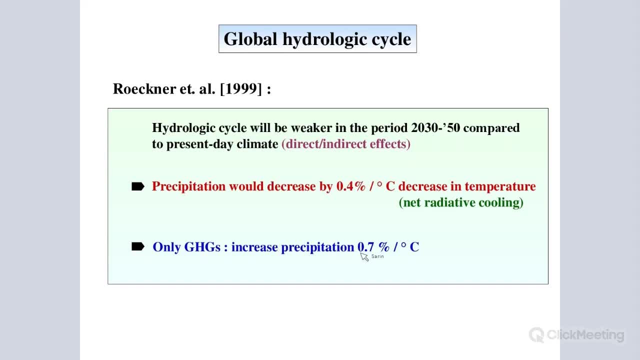 have net, net cooling on the on the system, and then the only greenhouse gases are going to to have the increased precipitation void by 0.7 percent per degree centigrade. so what the the message which which is this study is trying to give is that the greenhouses gases are going to have 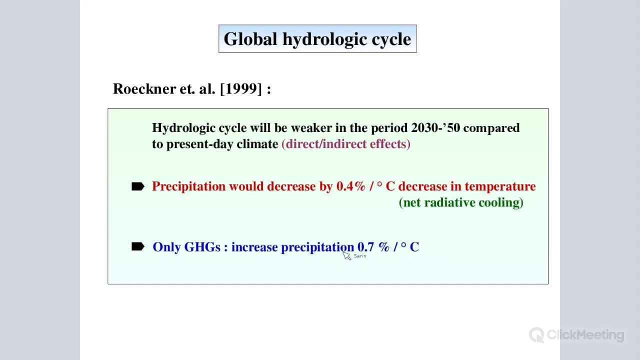 the warming potential in the atmosphere. they are going to increase the precipitation. so if we do not have the anthropogenic aerosol, we will have the increase in the precipitation by 0.7 percent. particularly this is what uh people have been talking about, that the uh in the, in the, in the 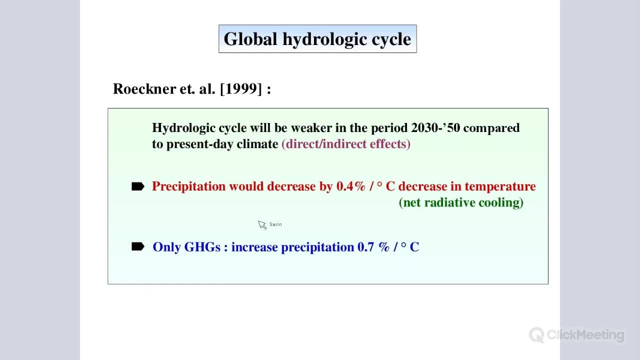 global warming scenario, you will have more of precipitation, but if we have the, the precipitation can decrease because of the, of the impact on the air from the aerosol. so you will have a decrease in the in the precipitation, and which is largely because of the of the decrease in the in the 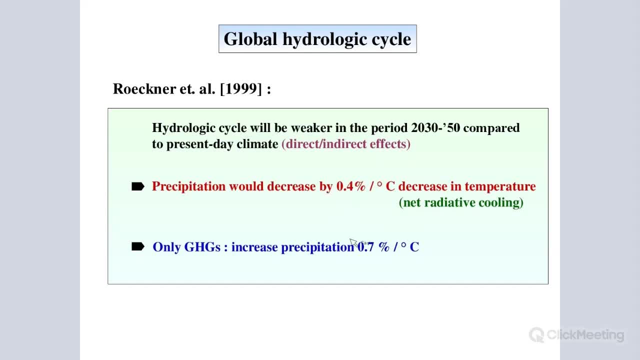 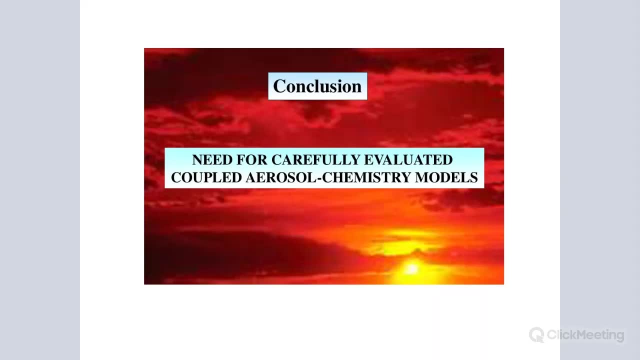 temperature and coming from the coming from the aerosols. so this is something which is important in the, in the climate change. so in. finally, i would conclude that the there is a need for very carefully evaluated coupled aerosol chemistry models. so which is what? so not only we. 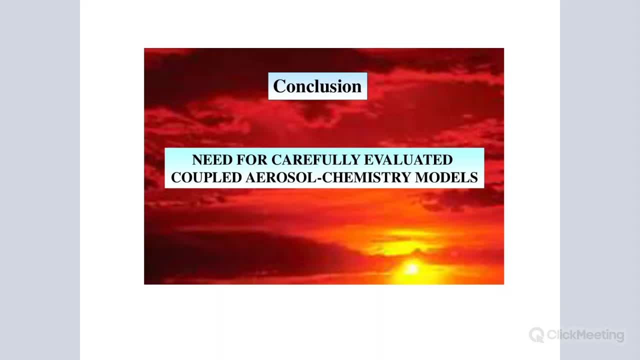 need the model, but we need the, uh, the chemistry built into the, into these models and- and that is something which is uh important in the, in the scenario, to understand uh, the, the cooling effect due to aerosol and the warming potential from the greenhouse gases. so there is a